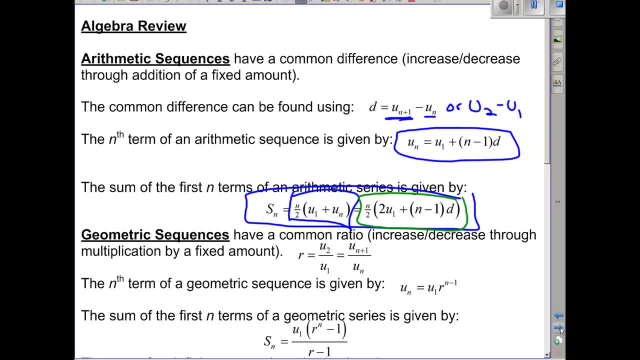 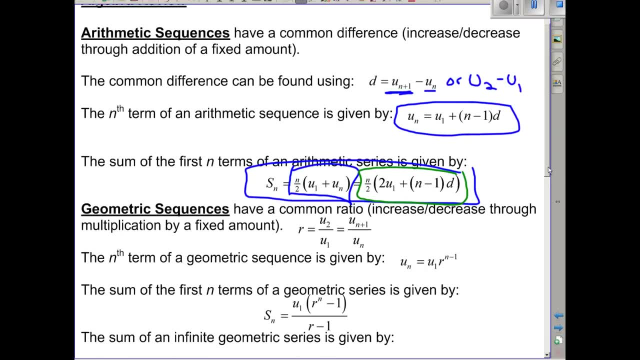 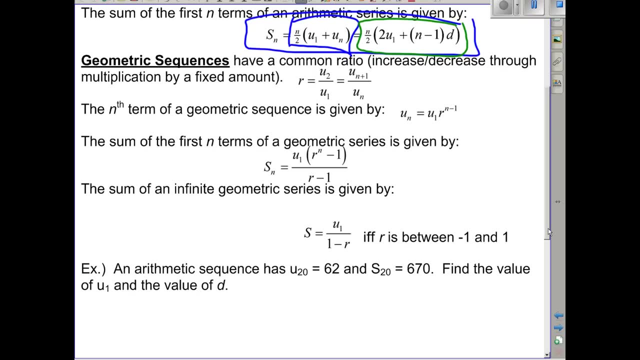 This one over here is great, if you know n the number of terms, the first term and the common difference. Geometric sequences have a common ratio. That means they increase or decrease by multiplication by a fixed amount And that fixed amount is called that common ratio. 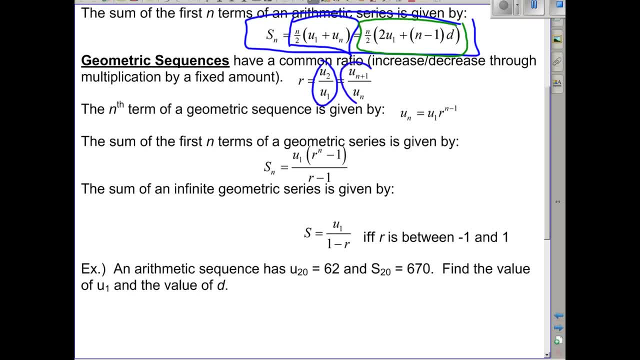 It's given by the second term divided by the first, or generally the n plus 1th term divided by the nth term. So if I have a sequence that goes 3, 12, 48. It seems like I'm going up through multiplication here. 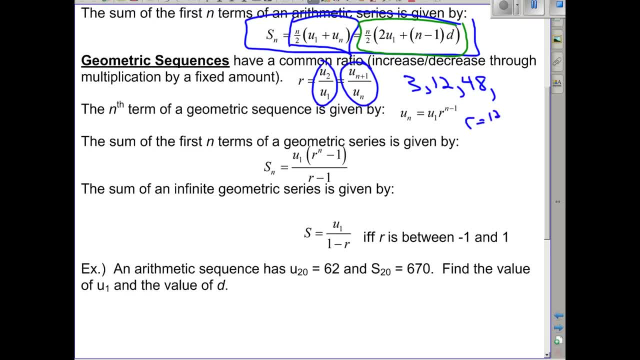 The common ratio would be 4, which I could find by 12 divided by 3, gives me 4.. And I can verify, because the third term, divided by the second, is also 4.. Or 48 divided by 12 is 4.. 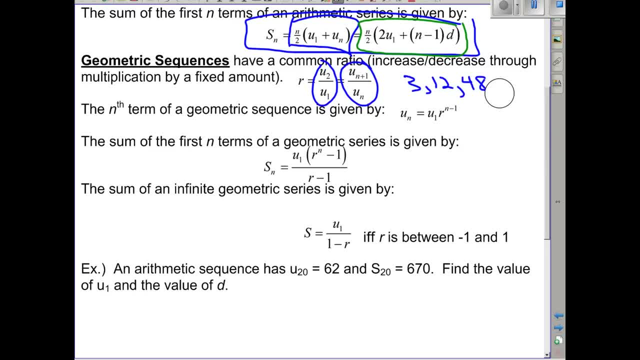 So the common ratio in that case would be 4.. Now let's consider a geometric sequence that goes, I don't know, say the other way around: 48,, 12,, 3.. Here you might be tempted to say I'm dividing by 4 every time. 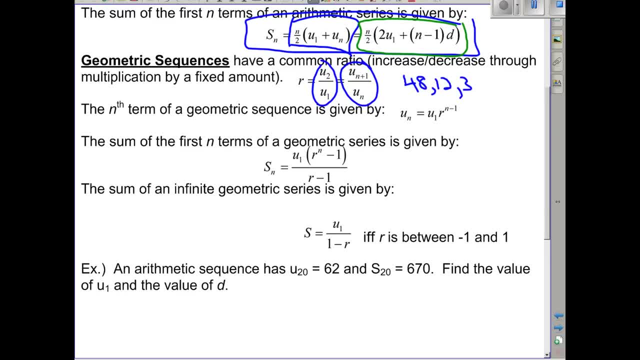 But common ratios need to be framed in terms of multiplication. So instead of saying I'm dividing by 4, let's say I'm multiplying by a quarter, And that could be shown by second term divided by first term, which is a quarter or 0.25. 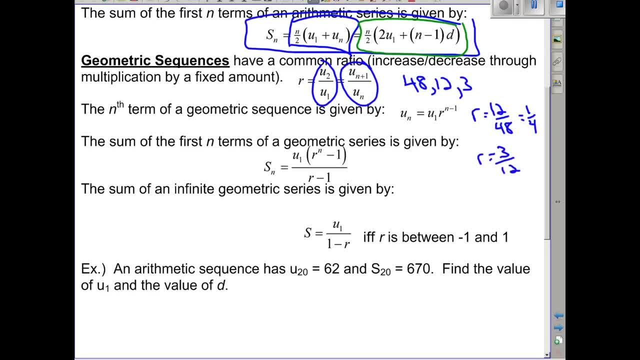 And verified by third term. divided by second, 3 over 12, that's still a quarter. Okay, So we're showing, We're showing here that it's a ratio and that it's common. It stays the same throughout the sequence. 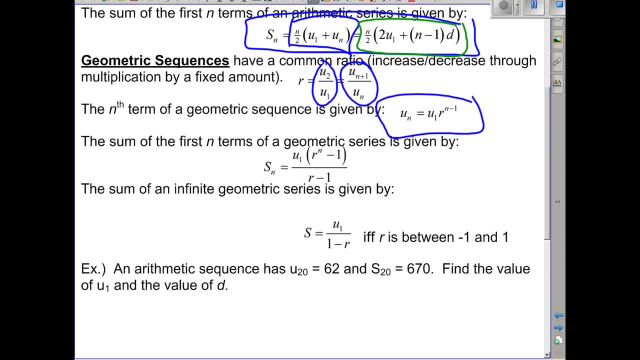 The nth term is given by this statement. here First term times the common ratio to the power of n minus 1.. The sum of the first n terms is given by this statement, And sometimes geometric series have an infinite sum. So if they go on forever and ever, they're actually going to converge on a number. 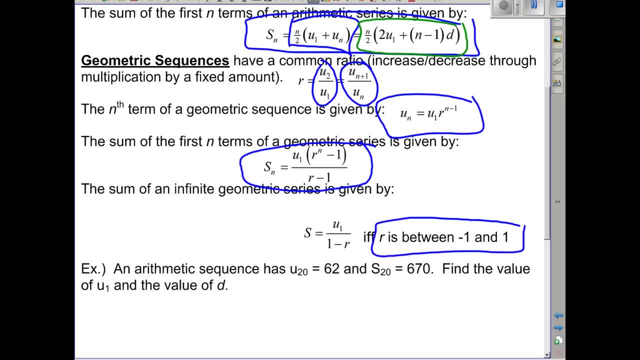 And that happens if your common ratio is between negative 1 and 1.. And that sum is given by u1 over 1 minus r. Okay, You could also call it negative u1 over r minus 1.. That would also work out. 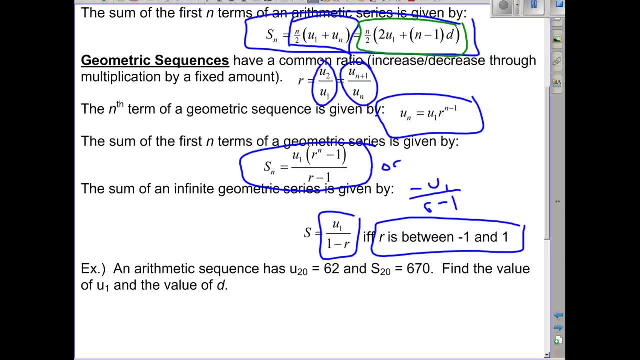 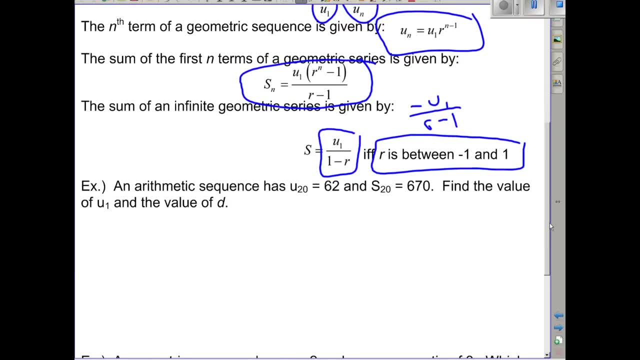 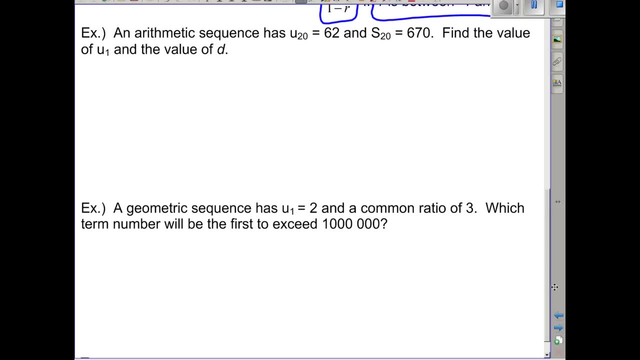 And there is also another formula that you could use for the Sn, which is in your formula booklet. Okay, Arithmetic sequence. Let's take a look at A fairly straightforward problem here. Has a 20th term of 62. And the sum of the first 20 terms is 670.. 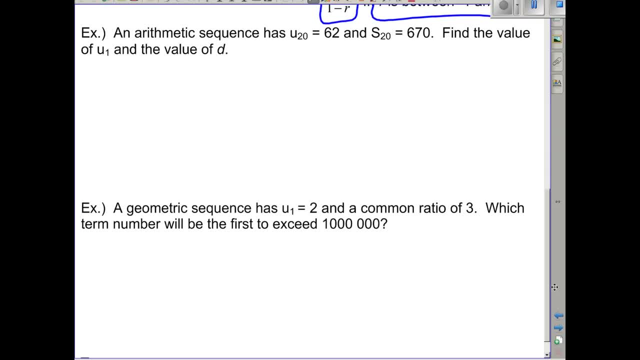 Find the value of u1 and the value of d. Well, in both these cases, here we're talking about n being 20.. So essentially, we know the 20th term, the sum of the first 20 terms and what n is. 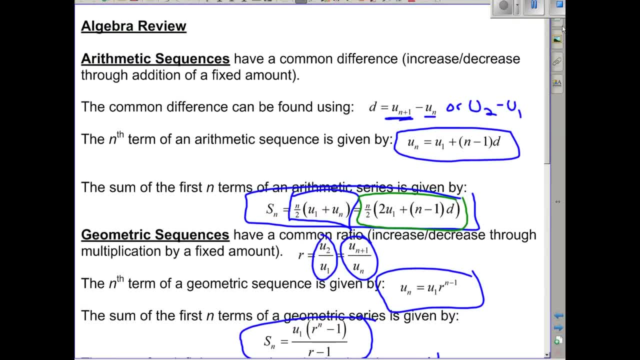 Let's see if there's a formula for sequences and series, for arithmetic situations, that uses those, Those, Those Bits of information. So we know n- Yeah, that's good, I know Sn And I know the nth term. This formula right here seems like it would work out well for us. 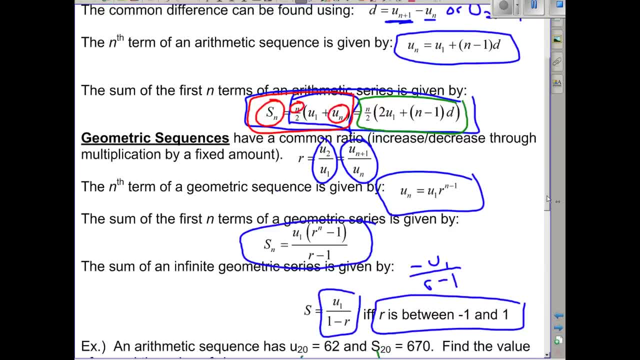 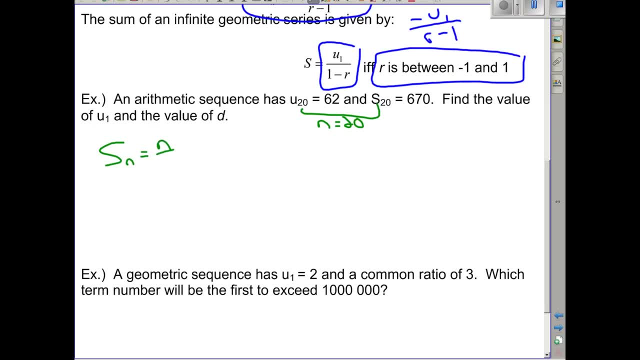 We could solve for u1 because there's only one unknown left. There are other ways of approaching this. I think this is probably the fastest one. Not n over 20.. n over 2. u1 plus un: Okay, substitute in what we know. 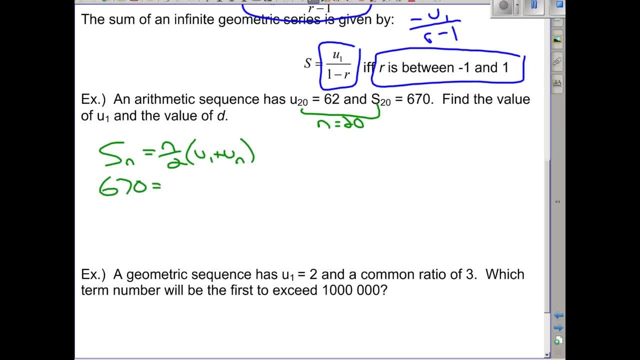 Sum of the first 20 terms is 670.. n is 20.. u1 is unknown And un or the 20th term in this case is 62.. 20 over 2 is 10 times u1.. And also 10 times 62.. 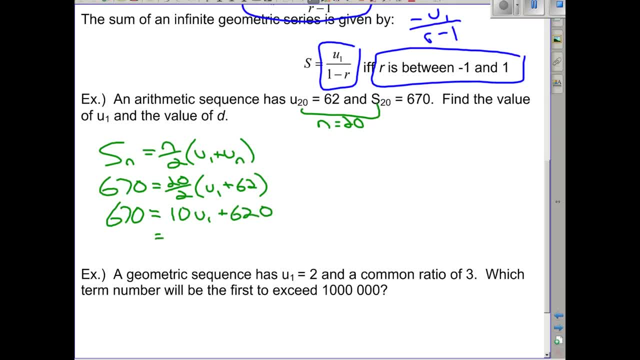 Which would be 620.. We'll solve here. We have 50 equals 10 times u1. Or u1 equals 5.. Great, We've found the value of u1.. Now we want to find the value of d. 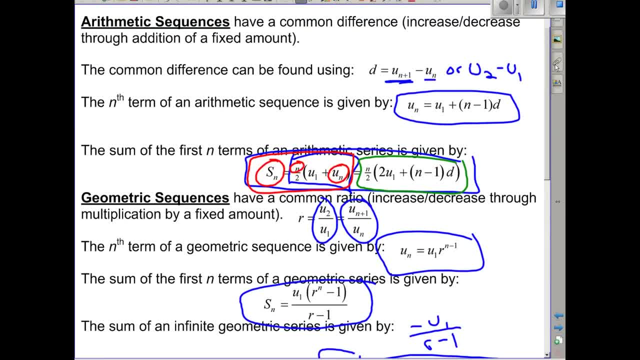 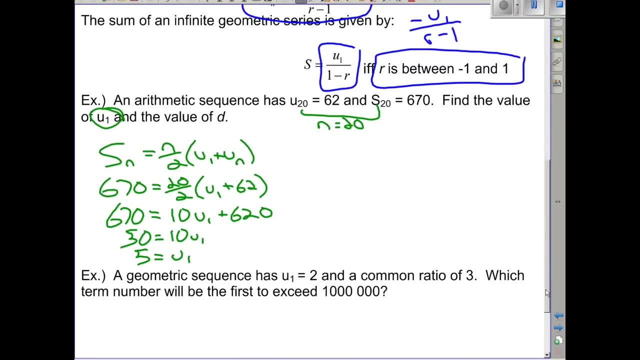 We could use either the Sn formula that has d in it, Which would be this green one up here, Or we could use our un formula. Well, we definitely have to use a formula that comes from arithmetic sequences and series, not geometric. Okay, so I'll take a look at the rest of this. 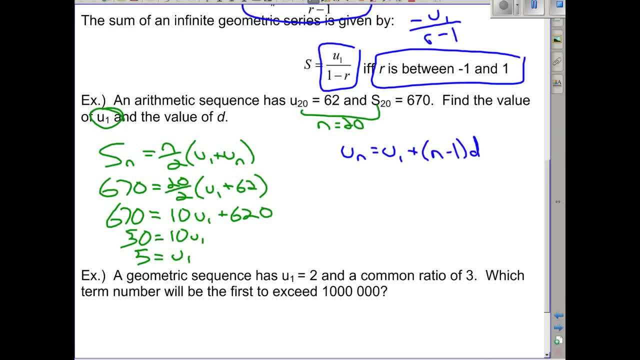 un equals u1 plus n minus 1 times d. Plug in what I know: un, the 20th term is 62.. u1, I know, is 5, now n minus 1.. I'm talking about 20 minus 1.. 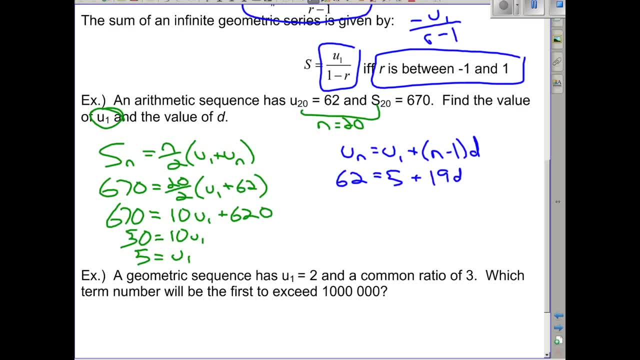 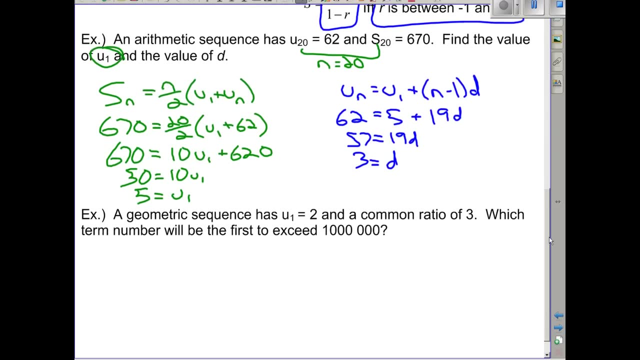 Because 20 was our n, So this would be 19.. Solve and I get 57 equals 19d, Or d equals 3. So I'm just cataloging what I know in these cases and plugging in to a formula that will. 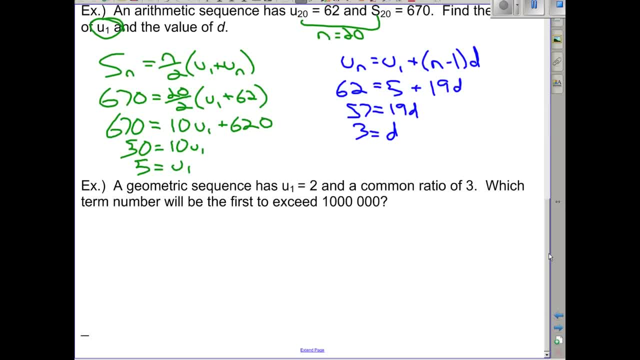 allow me to solve the question that's being asked, Namely find u1 and d in this case. Let's take a look at a geometric sequence. It has u1 of 2 and a common ratio of 3.. We want to find out which term number will be the first to exceed a million. 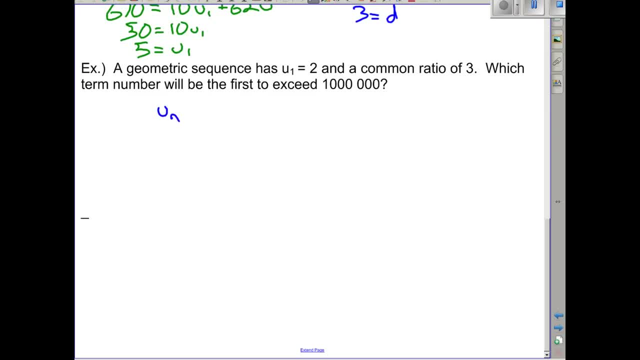 Okay, so that means we're going to use our geometric sequence formula: un equals u1 times r to the n minus 1.. Let's plug in what we know here. We know that our u1 is 2. That our common ratio is 3.. 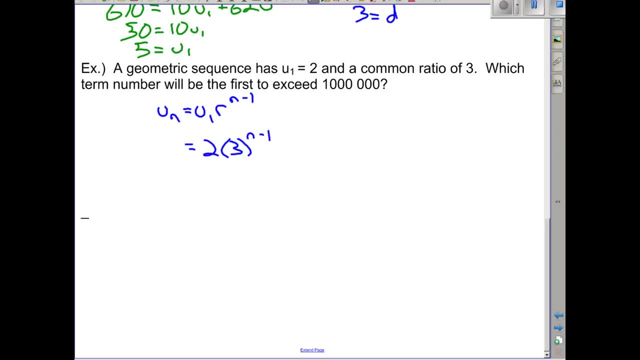 We're looking for the term number, which would be n, And actually we want to use our geometric sequence formula. Let's plug in what we know here. We know that our u1 is 2. And that value to exceed 1 million. 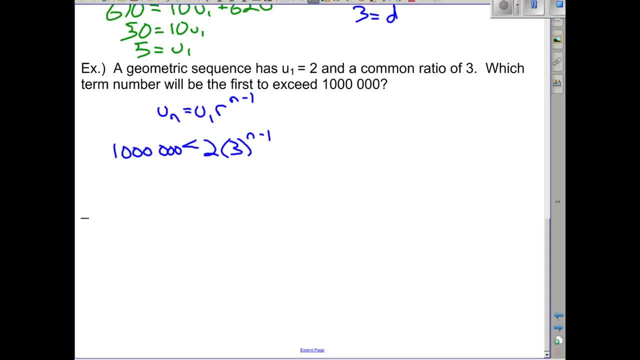 So if I read this from left to right, from right to left, it's saying 2 times 3 to the n minus 1 is greater than a million. Now we could solve a corresponding equation, Okay, And there are a bunch of ways to solve that. 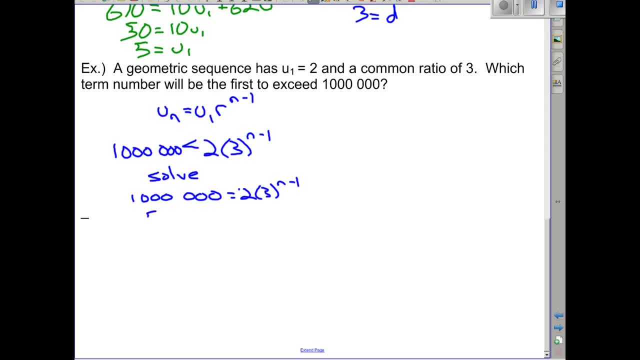 Okay, You can. first of all, you can divide by 2 and then use logs- Probably the most straightforward approach. Okay, Take the log, either base 10 or natural log of both sides. I'm going to take base 10, but it doesn't matter. 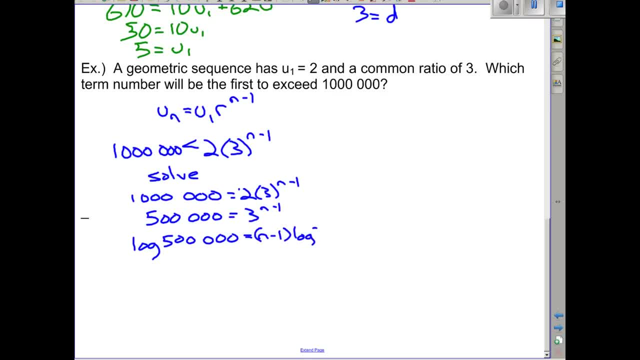 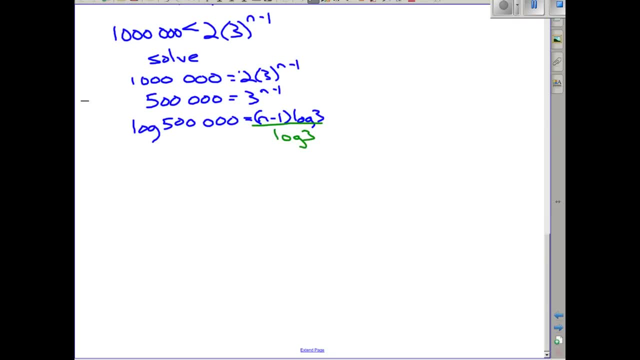 Bring down my n minus 1, my exponent as I do it, And then divide both sides by log 3.. Okay, Okay, Okay. So the goal here is to isolate n. Okay, Pull up my calculator Log of 500,000.. 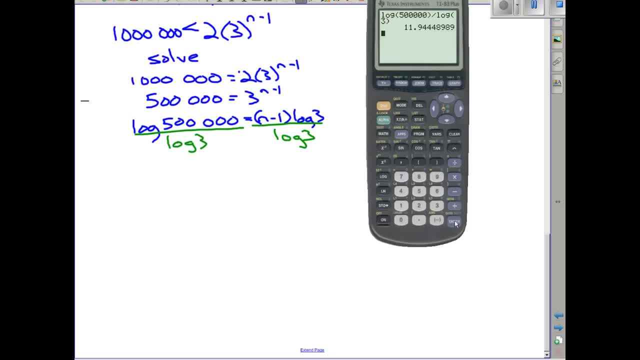 Make sure I close my brackets. Divided by log 3 equals 11.94.. And that would be what n minus 1 is, So n itself is going to be 12.94.. Just add 1 to each side. There is no 12.94th term. 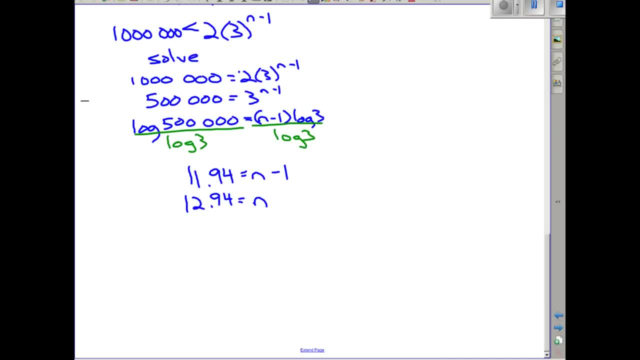 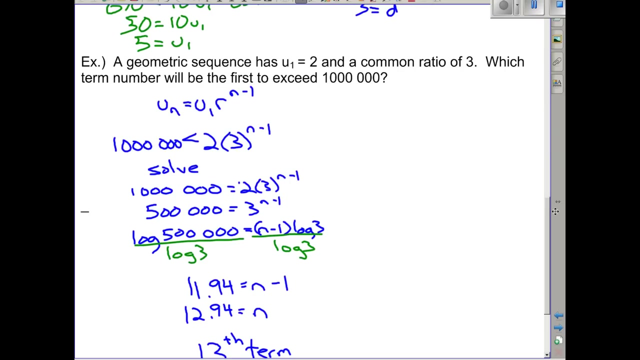 So we have to say here that it's going to be. since this is a geometric sequence that grows, it's got a common ratio greater than 1, we're going to be looking at the next term, the 13th term. Some other approaches to solving this might involve using your GDC to solve, say this: 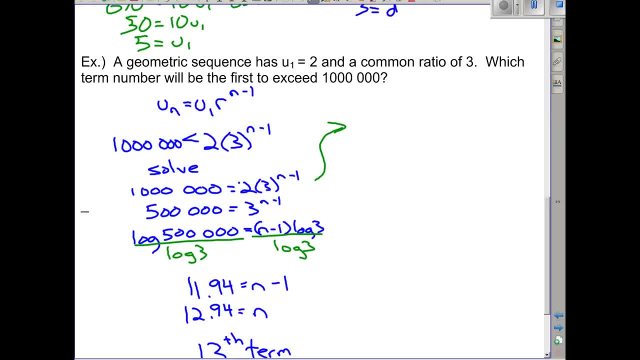 equation. Okay, So you could say that y1 is going to be 2 times 3 to the n minus 1.. I'm going to put that in my GDC: 2 times 3 to the power of x minus 1.. 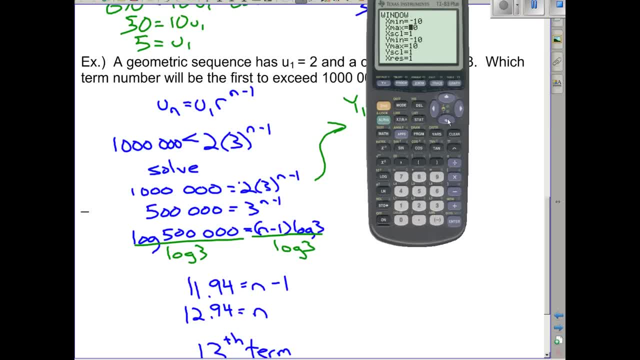 I could graph that. I know I want to see all the way up to what happens with a y value. Okay, I will start with a y value of a million, So I need to go up to at least a million. Maybe I'll go up a little higher. 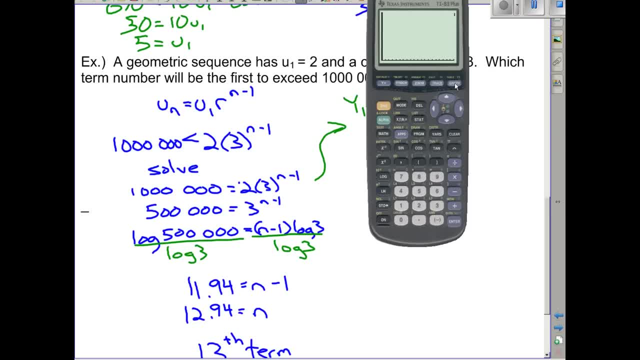 There we go. So somewhere around there I can figure out where it's going to be a million. I can put y2 in of a million and find that point of intersection. Okay, Right, Thank you very much. Thanks, Jeff. 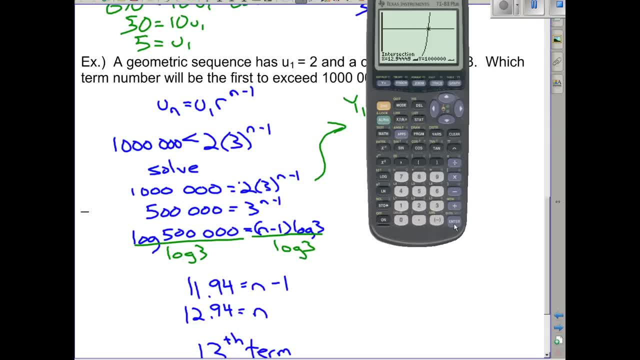 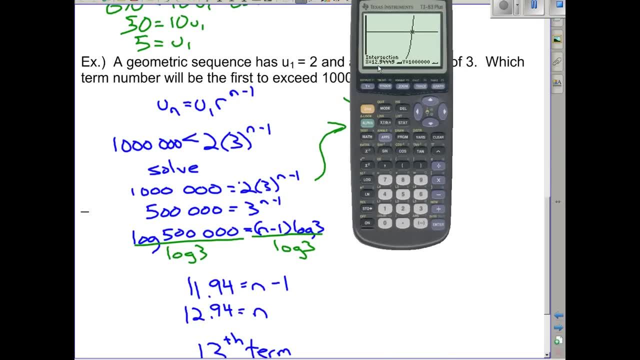 And it's going to give me x equals 12.94.. If I instead went to the tables and looked at what's happening for my y1 curve, I'll see that the 13th term is the first one to exceed a million. 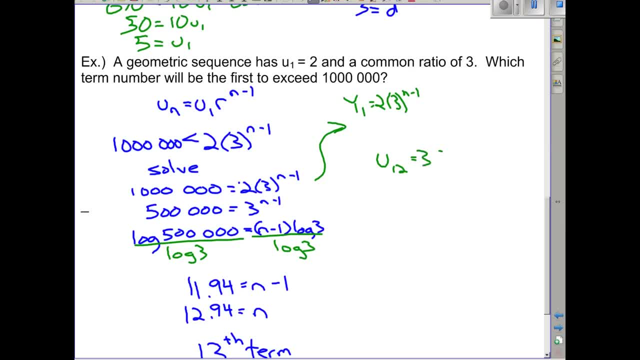 So I can show that u12 is from that little table- 354,294, and u13 is a million 62,882.. Whole bunch of different approaches here. I kind of like the logarithmic one best, but it's up to you. 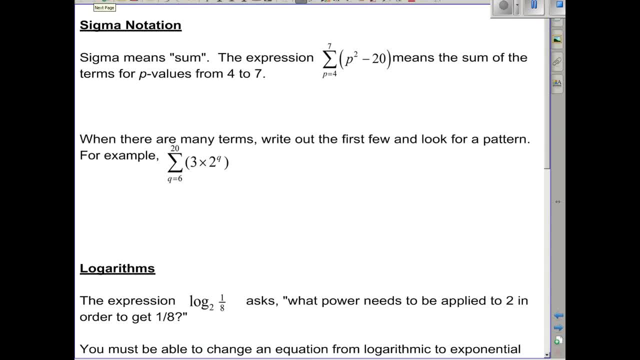 Okay, sigma notation. Sigma means the sum, And this is capital sigma, not to be confused with lower case sigma, which we're using for standard deviation. So the expression that's given means the sum for p values from 4 to 7.. 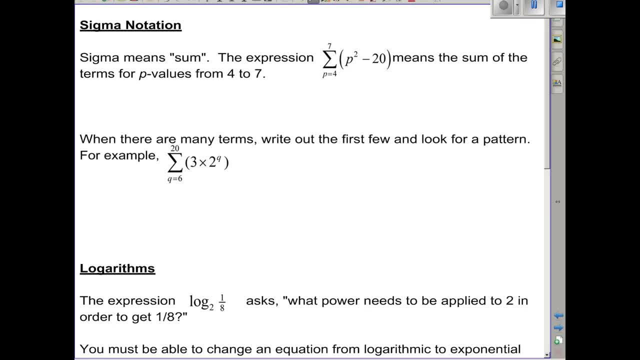 So all you really need to do here is substitute in those p values. If I put in 4 for p, I'll get 4 squared, which is 16, minus 20, or negative 4.. Then we're going to add on what we get when we put in 5 for p. 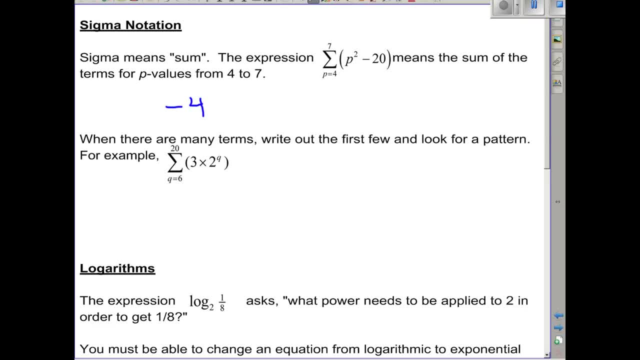 5 squared is 25.. Minus 20 gives us 5.. Put in 6 for p: Okay, so this was p equals 4,, this is p equals 5, p equals 6.. If I put in 6 for p, I'll get 36 minus 20, which is 16.. 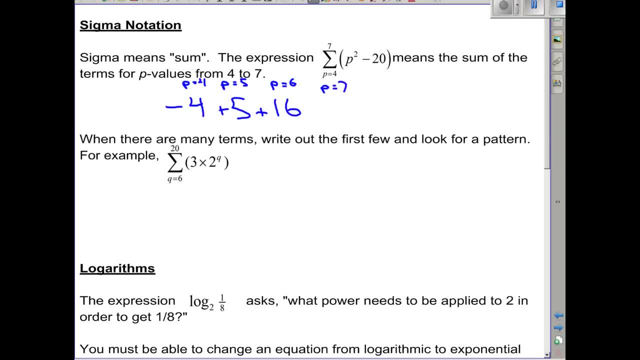 If I put in 7 for p, I'm going to get 49 minus 20,, which is 29.. Add them all up And the sum is going to be 49.. Okay, That's 36.. Now, often it's going to be really inconvenient for us to write out all of the terms. 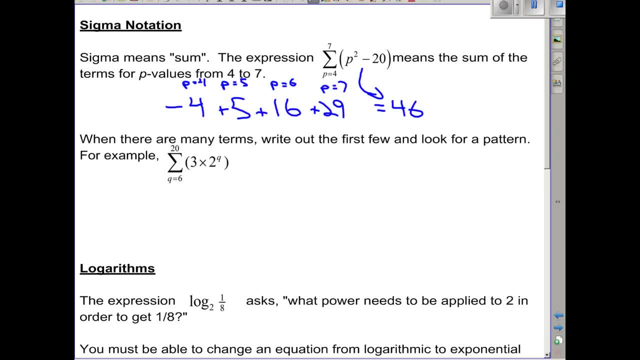 We'd have to write out the first few and just look for a pattern In the first one. no problem to write out those four terms and add them up, Probably the simplest way to approach it. All right, let's see what happens here. if we have from q equals 6 all the way up to 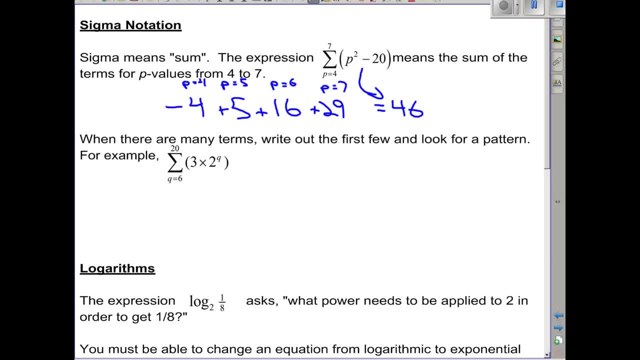 20, 3 times 2 to the power of q. So if I put in q equals 6.. I know that 2 to the 6 is 64 times 3 is 192.. Okay, Plus, what happens when I have q equals 7?. 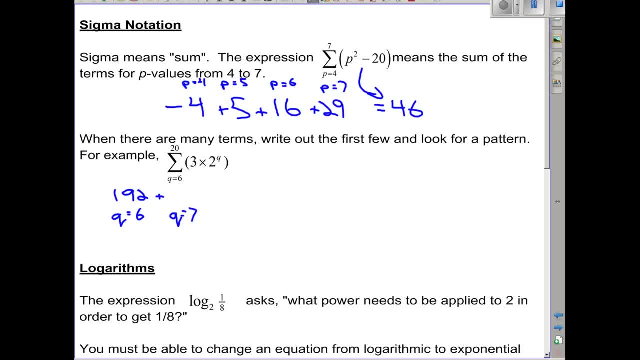 2 to the 7th is 128 times 3 is 384.. q equals 8.. Okay, That would be 256 times 3 or 768.. Hmm, And this is going to be a pain to keep writing. Now let's see what we have here. 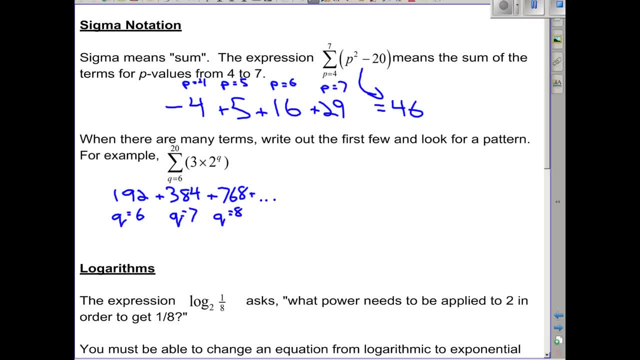 384.. 184.. 192.. Hmm, We seem to have doubled and then doubled again. This is a geometric series that we're showing here, So rather than write them all out and add them up, I can go to my geometric series. 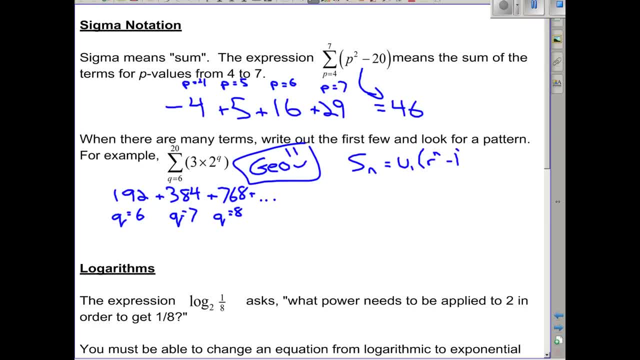 formula And this is the version of it I like to work with. Some people might use this one, which is also good. Okay, Can I change it? 10, okay, 10, now is a little bit faster, Makes no difference. 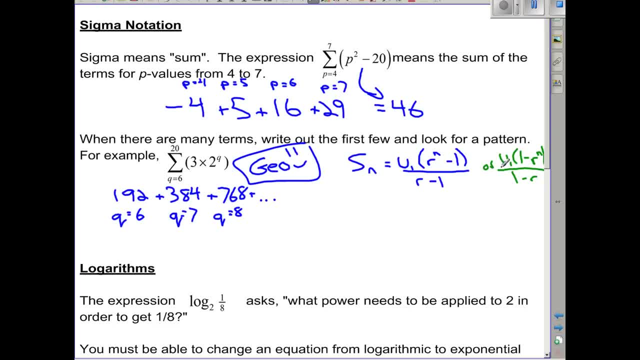 Okay, substitute in what I know Well I want from the 6th to the 20th terms: Hm, That's actually 15 terms, So I'm looking for s15.. The first term was 192.. The common ratio I'm going up by multiplying by 2's, so this will be 2 to the power of. 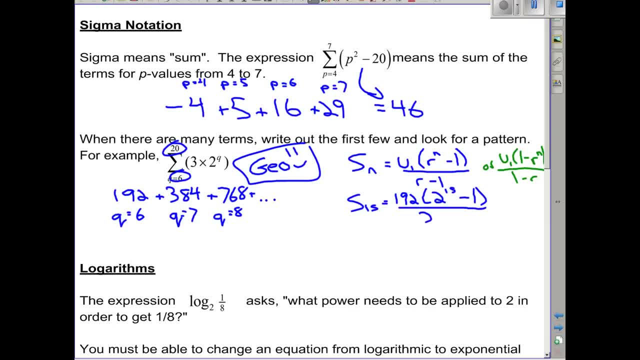 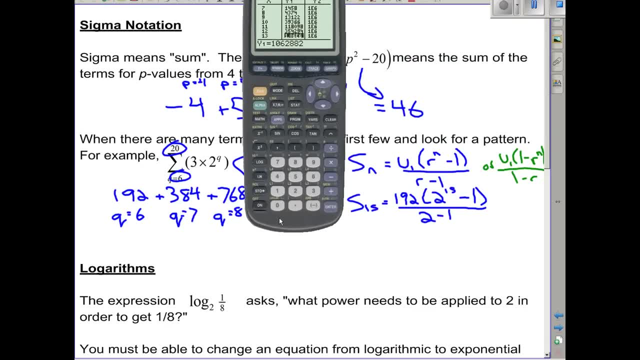 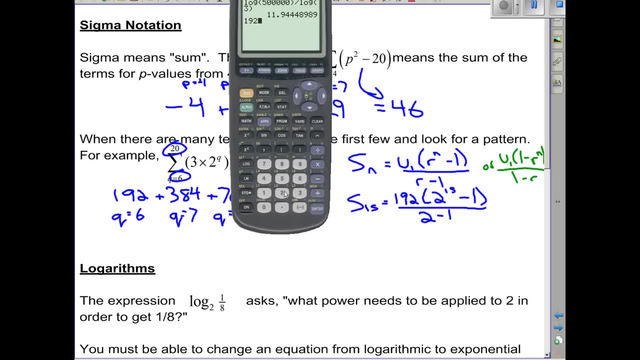 15 minus 192.. minus 1, all over r minus 1, so 2 minus 1.. I'll plug that into my GDC: 192 open brackets: 2 to the power of 15 minus 1 divided by. I really shouldn't have to put in 2 minus 1 in my calculator. 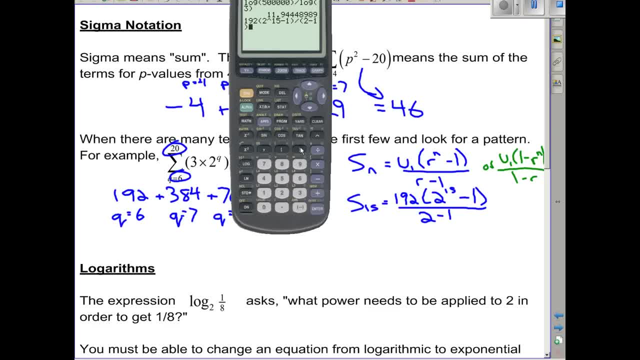 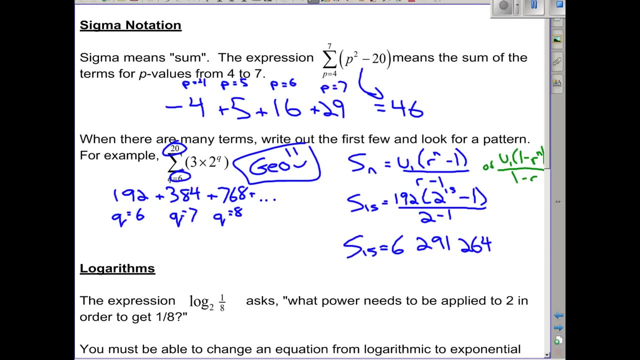 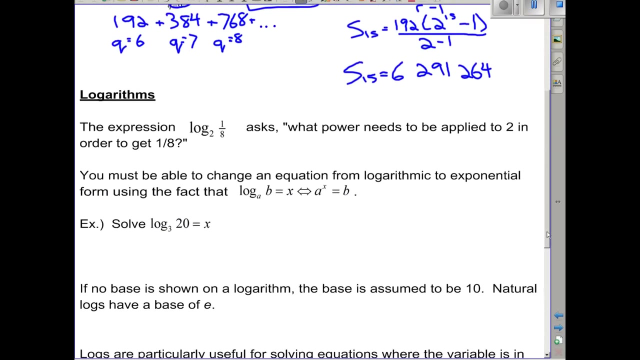 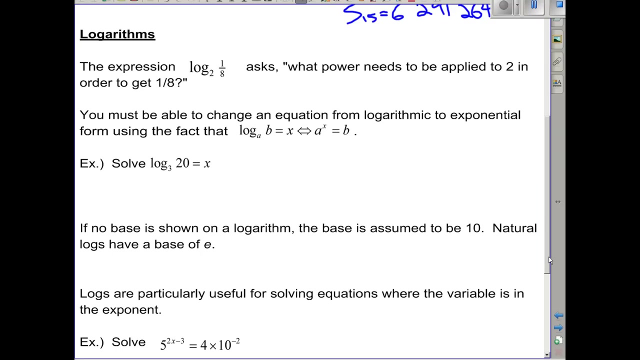 but I just want to show you to be careful of the brackets as you do it okay, and I should get 6,291,264. plug them in carefully. alright, logarithms. if you've got the expression log base 2 of 1, eighth, it's asking you a question. it's saying what power do you need to raise 2 to? 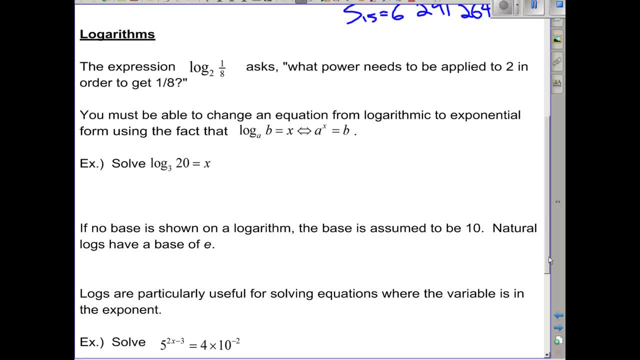 in order to get 1 eighth. So you know, 2 to the power of 3 gives you 8, and a negative power flips it upside down so that you've got a fraction. so the power that you need to apply to 2 in order to get 1 eighth must be a. 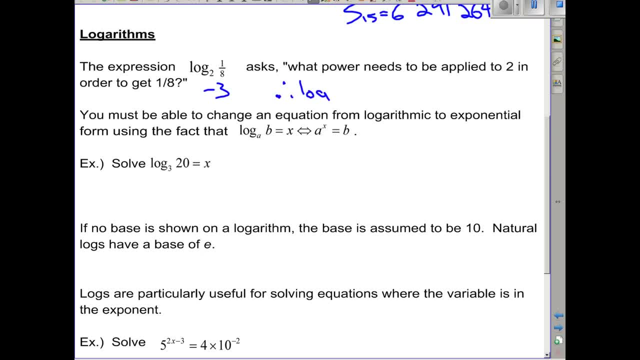 negative 3. therefore, log base 2 of 1 eighth is negative 3. it could also be written in exponential form, and in your formula booklet you're given how to convert between the two. in case you forget, I think this is the way it's written. 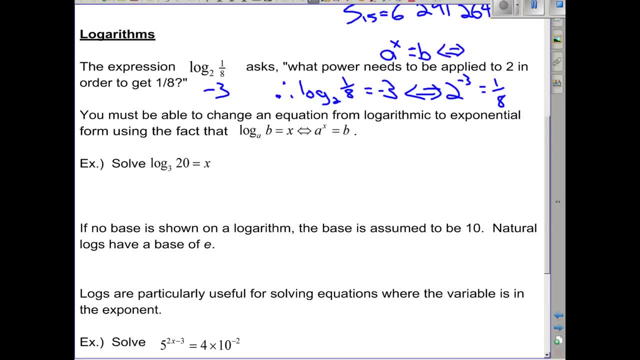 a to the x equals b can also be written as log base: a, b equals x. that's from your formula booklet. you need to be able to change an equation from logarithmic to exponential form and there I have it written using this fact. So if I've got log base 3 of 20 equals x, I can convert that into exponential. 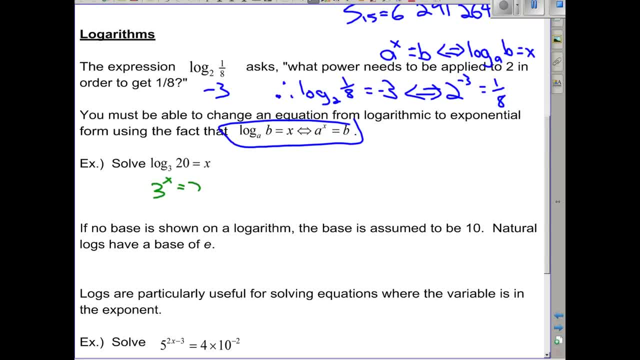 form: The base is 3, the exponent is x and the result is 20.. At this point I can take the log of both sides, either base 10 or natural log, So I can go log of 3 to the x equals. 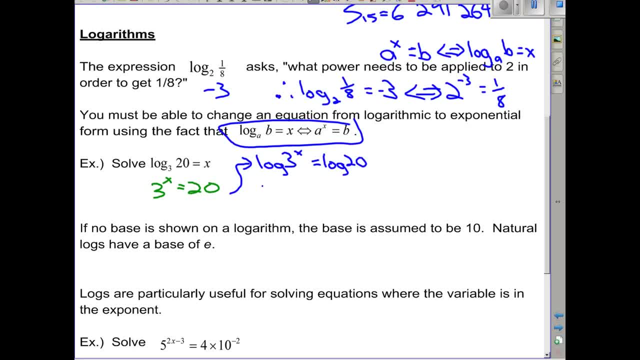 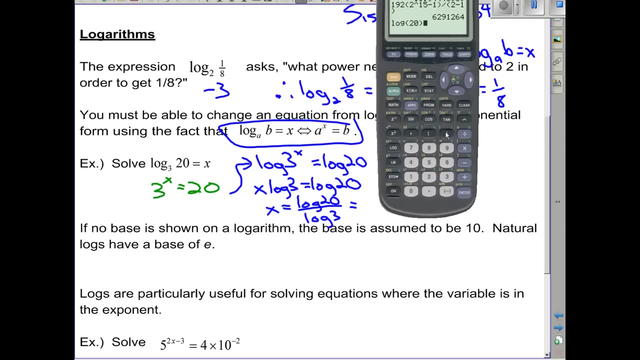 log of 20.. That lets me bring my x down and I can divide both sides by log 3.. We're just following the golden rule of equations here: Whatever you do to one side, you can also do to the other. So log of 20 divided by log of 3.. 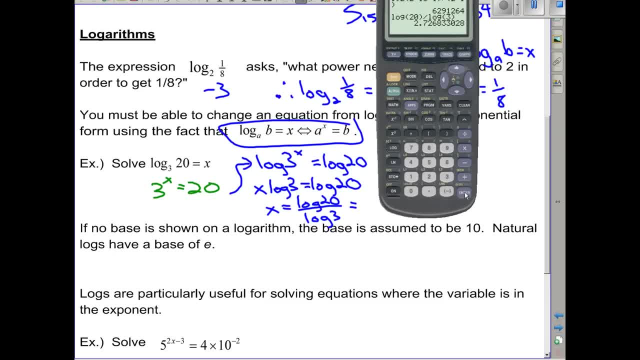 Can I go back and do that again? Can I go back and do that again? Can I go back and do that again? That's going to give us 2.73 to 3 sig figs. There's also a change of base rule which we'll look at on the next page. that simplifies. 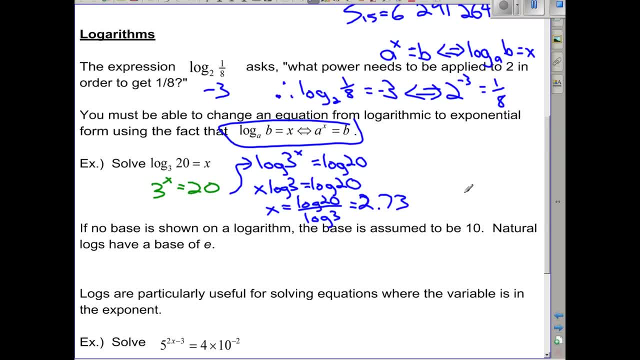 these types of questions. We could also check this. Put it back in Check- whether 3 to the power of 2.73 really does give us 20.. 3 to the power of 2.73.. Yeah, it gives us 20, with a slight rounding error. 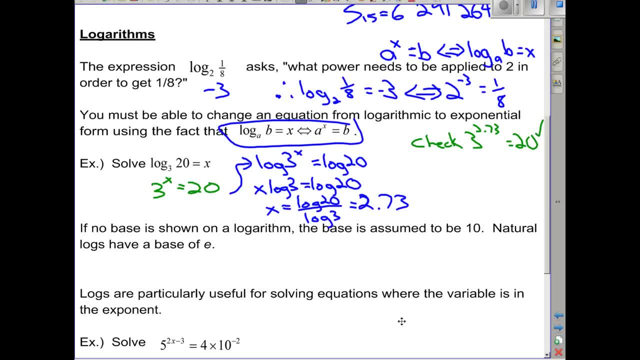 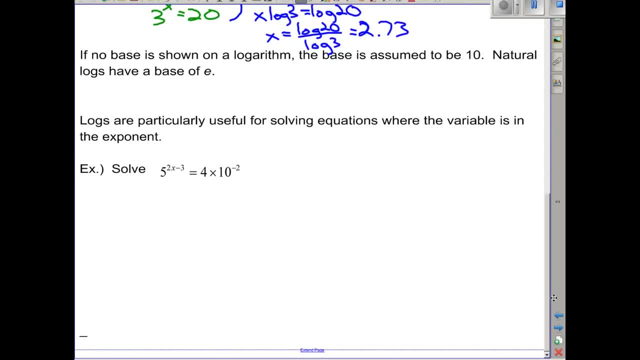 If no base is shown on a log, the base is assumed to be 10.. Natural logs have a base of e. Logs are great when you're solving equations where the variable is in the exponent. They let you bring it down using some of your log laws. 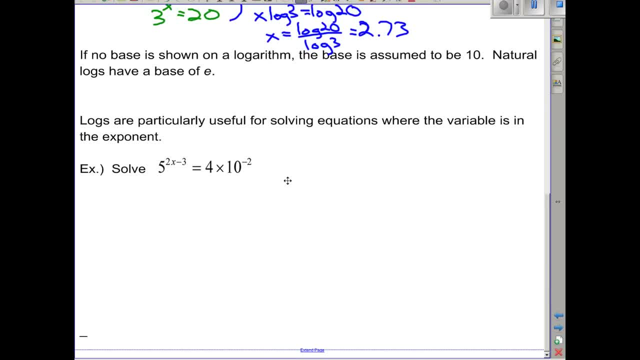 So if I had this equation right here, 5 to the 2x minus 3 equals 4 times 10 to the negative 2.. I think this actually does come from one of the old IB questions. My first inclination here would be to rewrite the scientific notation part as a decimal. 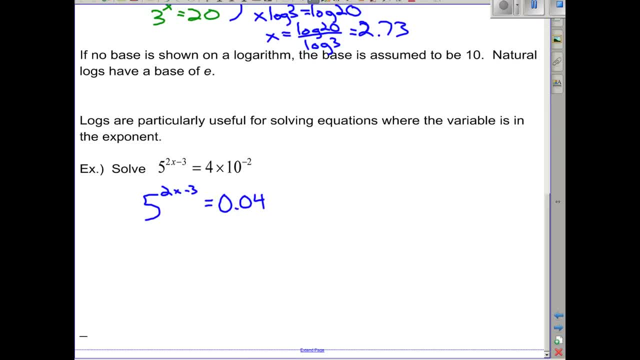 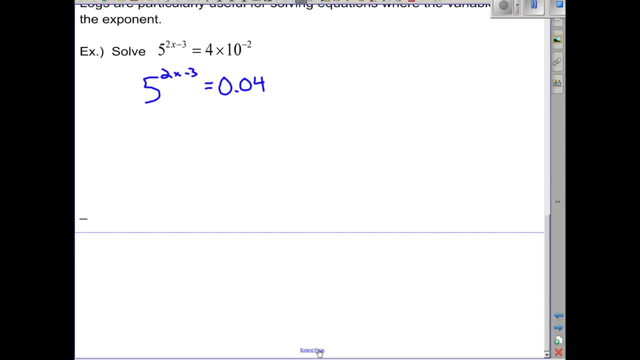 Though you can certainly deal with it in scientific notation. Alright, then we realize our variable is in the exponent. I'm going to need to take the log of both sides so that I can eventually bring that down. So log both sides of 5 to the 2x minus 3 log of 0.04.. 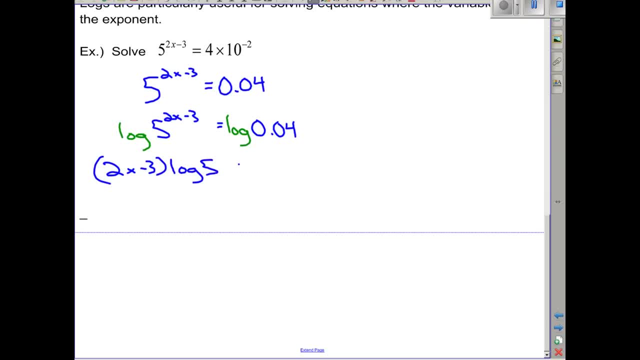 I can now bring down my exponent all together. I need to put it in brackets: Equals log of 0.04.. Divide both sides by log 5 to start isolating our x, So I'll get 2x minus 3 equals. 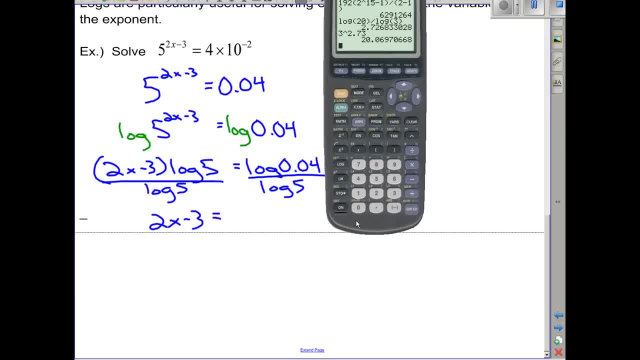 I might be tempted to go to the calculator at this point rather than wait until the very end. Log of 0.04 divided by log of 5 gives us negative 2.. Hmm, that's nice and convenient. It's not always going to work out that nicely. 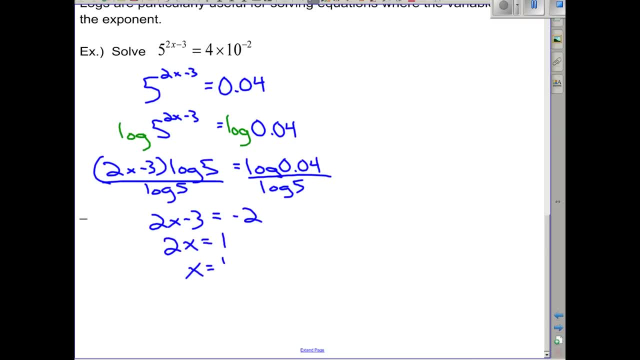 Gives us 2x equals 1 or x equals a half, And we could go back. We could go back and check that. Now you might be saying I had another way of doing it. Here would be an alternate approach. If you realize that 0.04 is the same as 1, 25th. 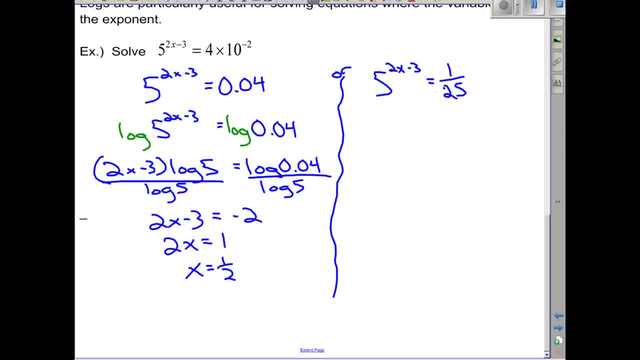 We could write it this way, Which initially doesn't look like it's helping out a whole lot, But then we say, okay, well, 1 over 25, that's 5 to the power of negative 2.. Ah, I've got it. 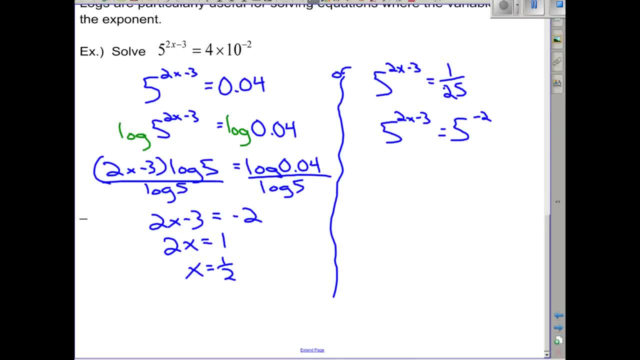 5 to the 2x minus 3 equals 5 to the negative 2.. When we have the same base on both sides- and we know that both sides must be equal- that means we must have the same exponents on both sides as well. 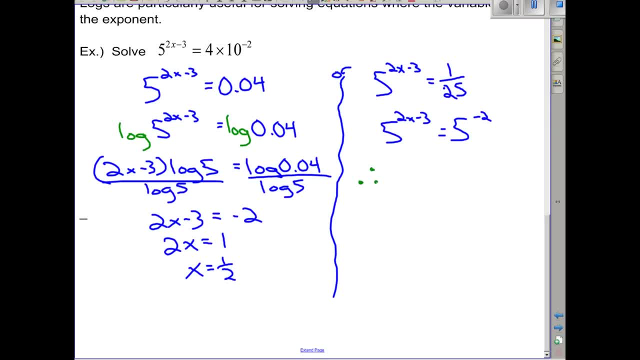 So I can equate my exponents: 2x minus 3 must equal negative 2. Which gives us 2x equals 1 or x equals a half. Didn't have to use my calculator at all to use that method. Ah, so, if you can find it, 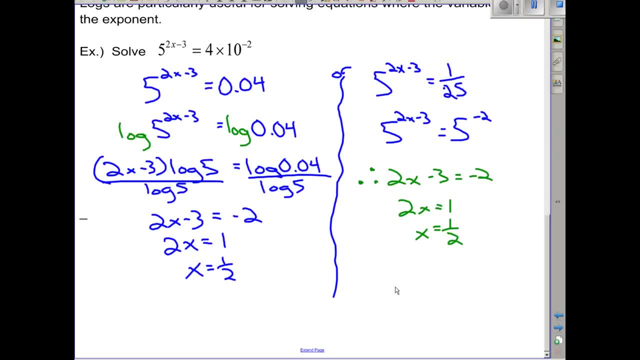 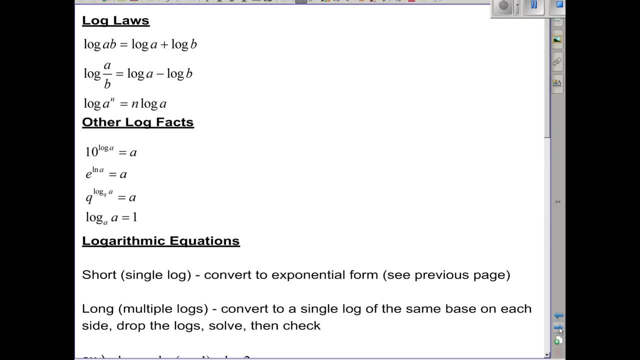 If you have a common base on both sides, the logs really aren't necessary. Let's take a look at our log laws. I didn't show any bases here, so they're assumed to be base 10. But they'll work for any base. 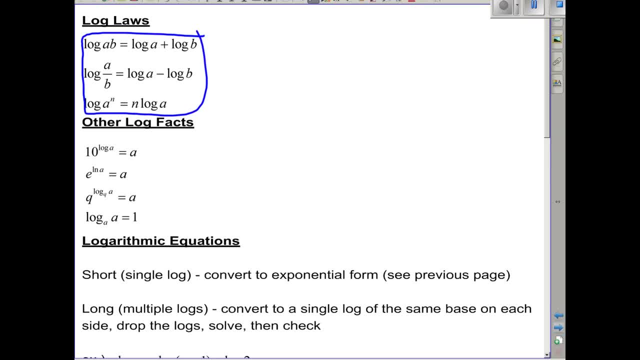 So log of ab is the same as log a plus log b, Log of a over b is log a minus log b. And this one right here tells you that you can bring your exponent down. And that's what we've been doing, Ah, in the last few questions. 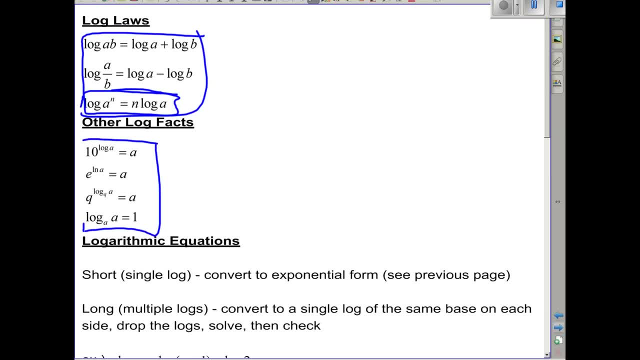 Okay, a few other little log facts here. This one's really important Log base a of a is 1.. So log base pi of pi is 1. Because it says what power do you have to raise pi to in order to get pi? 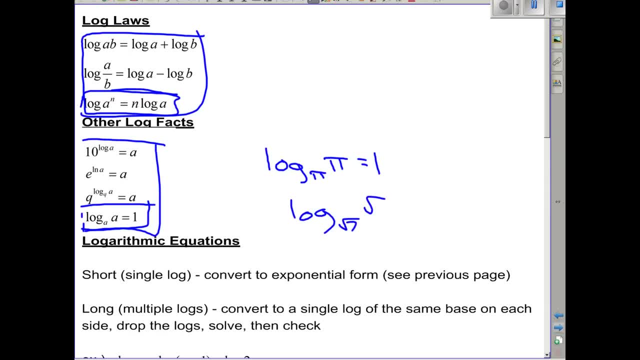 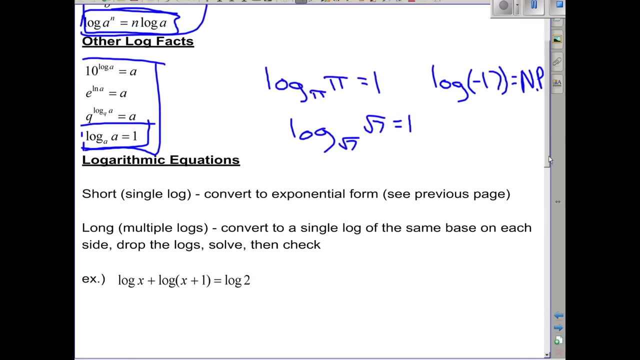 Log base: root 7 of root 7 would also be 1.. You can't take logs of 0 or a negative number, So log of negative 17, not possible. Okay, log equations. The way that I think of these is as following into two types. 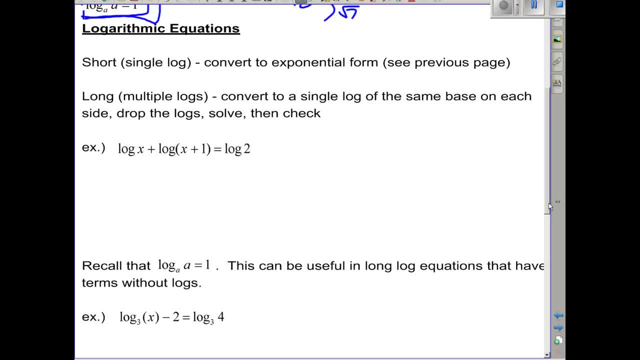 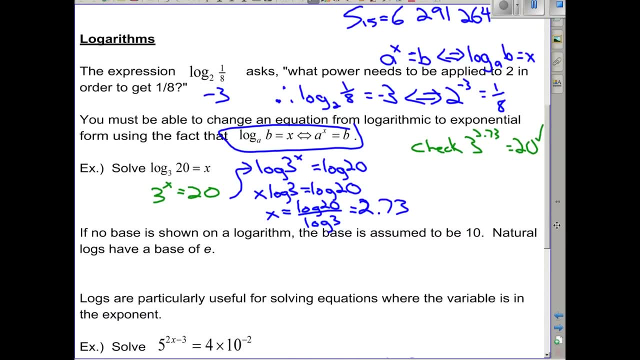 Short log equations would be ones that only have a single logarithmic term in them. Okay, so this one from the last page where we said log base 3 of 20 equals x only had a single log in it. We can convert it to exponential form and then use our logs to solve. 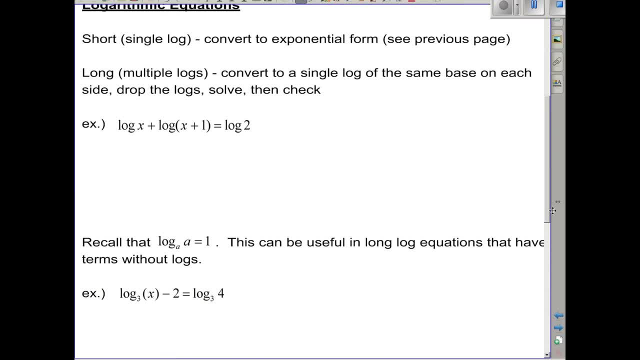 And then there are the types that I call long. They've got multiple logs. They're not more difficult, They just take a little longer to do Convert to a single log of the same base on each side At that point, just like we dropped the bases in the last question. 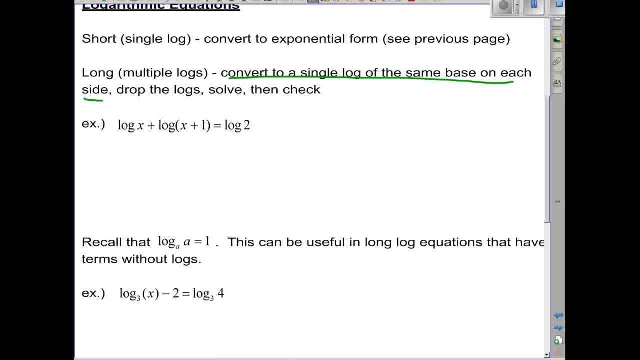 you can drop the logs here, You can solve, and then you need to check because you may end up with what's called extraneous solutions: Solutions that look like they work for the version of the equation that you're working with, but don't actually work in the original equation. 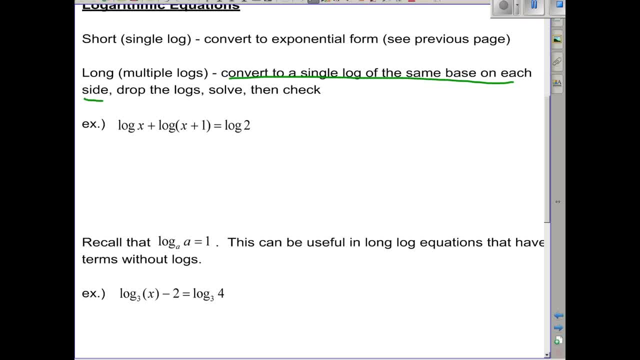 So for this one down here, we've got two logs on the left and one log on the right. We can put these together. Two logs being added means that you multiply whatever you're taking the log of. So x times x is x squared. 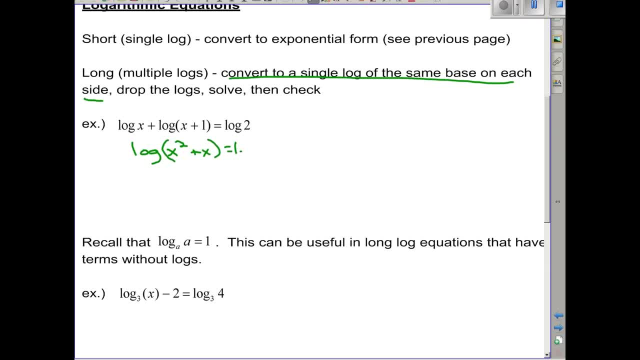 x times 1 is x. I put them together into a single log on the left and I already have a single log on the right. Now I can drop my logs- Ooh, it's a quadratic Factor- and solve What adds to 1 multiplies to negative 2.. 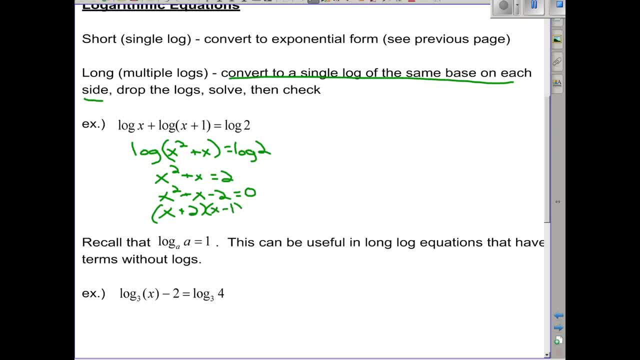 Oh, we can get plus 2 and negative 1, which gives us solutions of x equals negative 2 or x equals 1.. Now we go back. Let's go back and see if either of those cause a problem. If I put in x equals negative 2, back here. 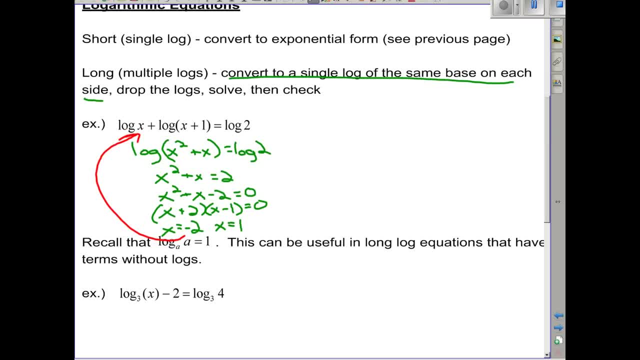 I'll be taking the log of a negative number. That is not allowed, So this is an extraneous solution. It doesn't count for our final solution. set The x equals 1, no problems, Log of 1,. I can do that. 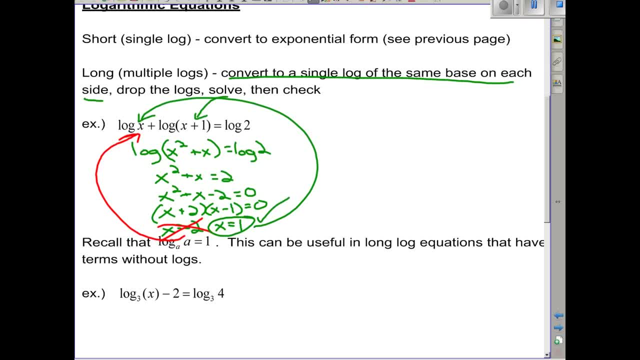 Log of 1 plus 1 or 2,. I can do that. This is our solution. So we only have one solution here of x equals 1, even though it looked like that, I think we might have two. Okay, recall that log base a of a is 1.. 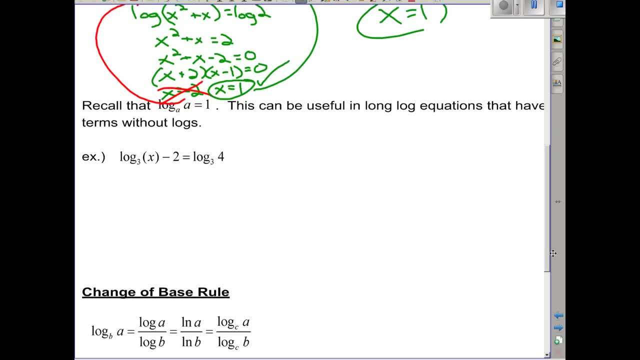 This can be helpful in a long log equation where you have one term that doesn't have logs. So over here I have log base 3 of x minus 2 equals log base 3 of 4.. How I would think of this is: this is 2 times 1,. 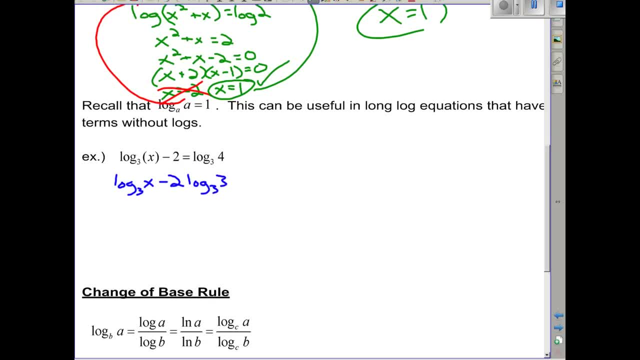 negative 2 times 1.. And another way of writing the number 1, is log base 3 of 3.. Now I can move that 2 up on top of the 3, because it's really an exponent that used to live up here. 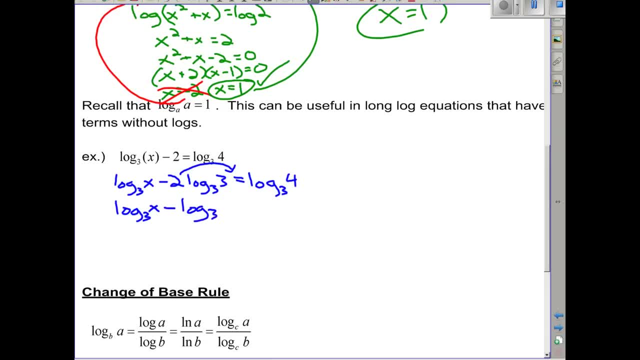 So minus log base 3 of 3 squared, which I might just write as 9.. And some people might have jumped to this step right off the bat. That's fine, Because they knew 2 is the same as log base 3 of 9.. 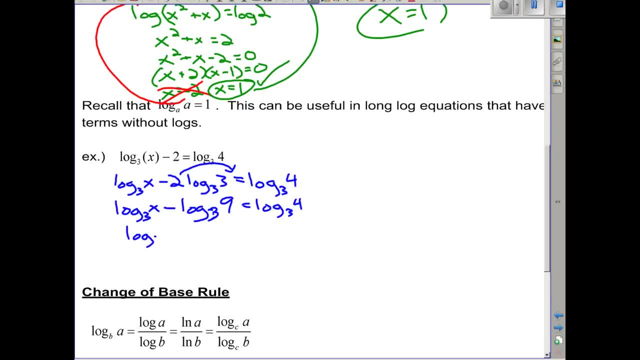 Okay, then that's going to give me log base 3.. I can put my logs together. on the left-hand side I'm subtracting logs, So I should get x over 9 equals log base 3 of 4.. Drop my logs. x over 9 equals 4,. 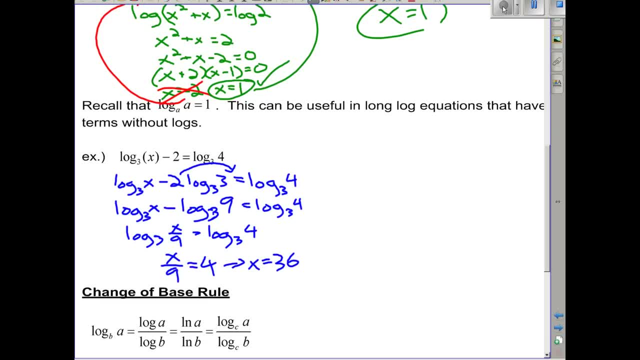 which in turn gives us x equals 36.. If I put that back in, I'd have no problems. An alternate approach for these kinds of questions, if that doesn't work well for you, would be to put all your logarithmic terms on one side. 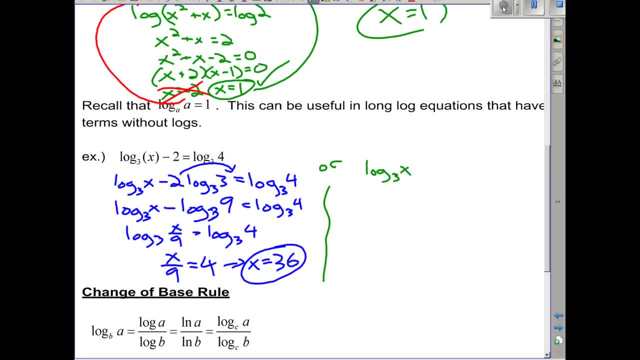 and put your regular numbers on the other, So you'd have log base 3 of x. I'm going to move that log base 3 of 4 over by subtracting it from both sides. I'm going to add 2 to both sides. 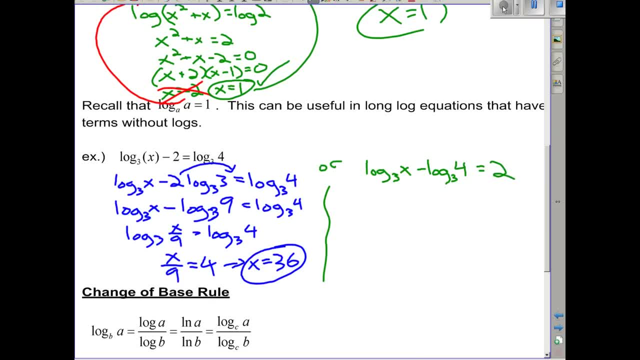 So I've just rearranged it in this format. Okay, I can put these together as log base: 3 of x over 4. And then treat it like one of those short logarithmic equations, Put it in exponential form. So I have a base of 3,, a power of 2, and a result of x over 4.. 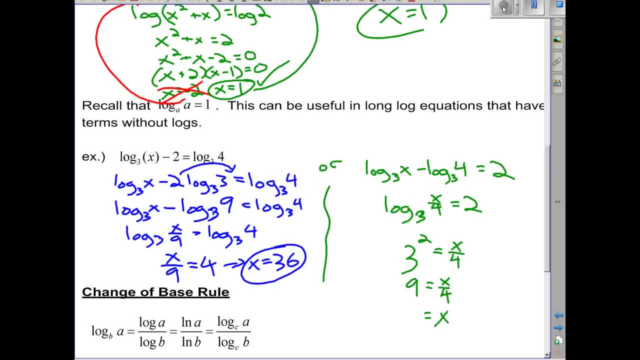 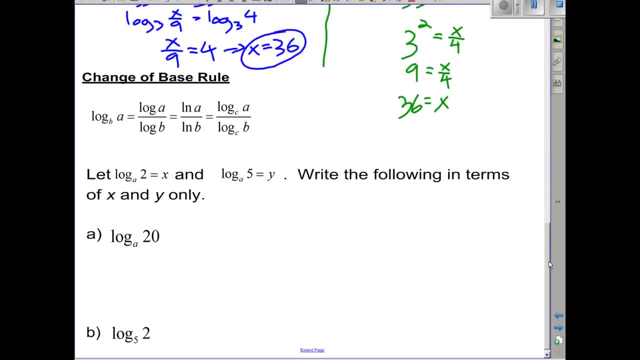 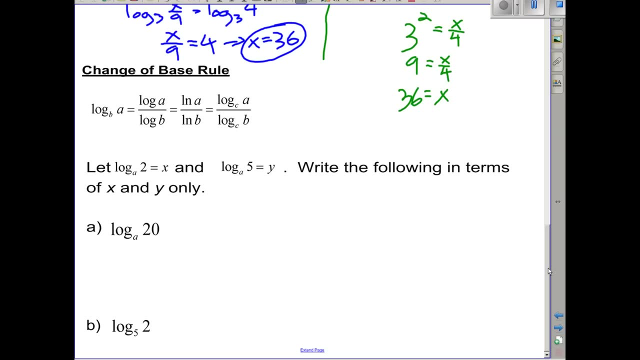 Gives me 9 equals x over 4.. Or still gives me x equals 36.. Either approach would be fine. Change of base rule: Log base b of a is the same as log a over log b Or ln a over log b. 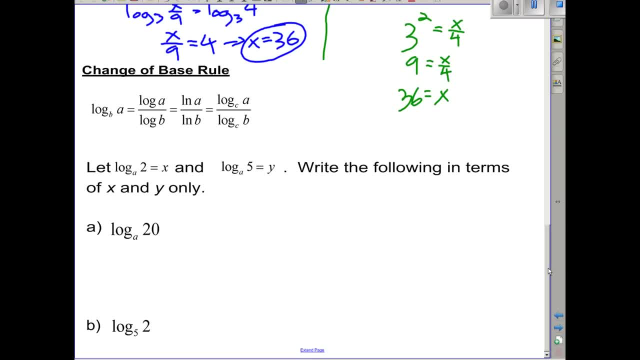 Or log with any base of a over log of that same base of b. So on the last slide we had done this Log base 3 of 20.. Change of base rule says that we should be able to do it as log 20 over log 3.. 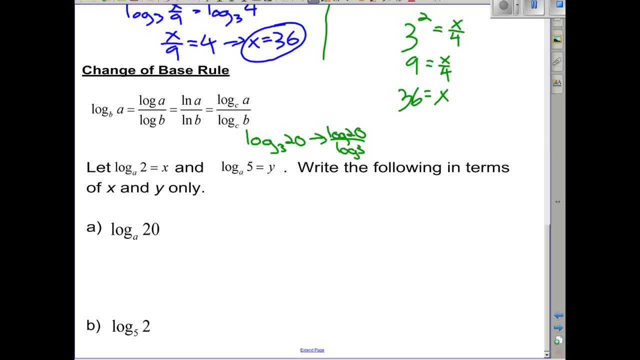 Which is what we ended up with, And we got 2.73.. Or we should be able to do it as ln 20 over ln 3.. Huh, I wonder if that works: ln 20 divided by ln 3.. 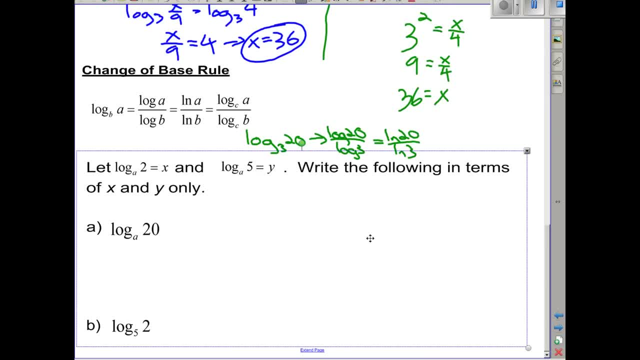 Yep works just as well, And if your calculator worked in different bases, you could do it in any number of bases. So the IB sometimes finds these great ways of testing you about these questions without using your calculator at all And keeping it somewhat abstract. 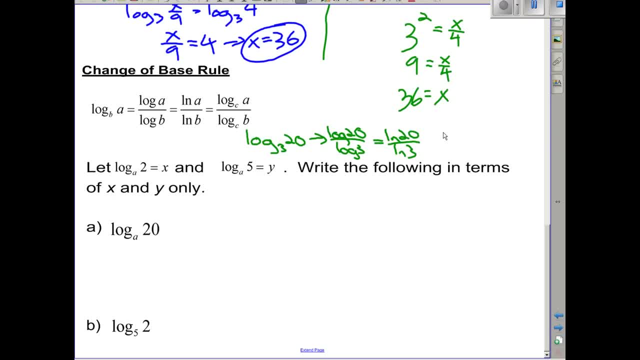 So this is a good case in point. Log base a of 2 is x. Log base a of 5 is y. Write the following in terms of x and y. only Now I know sometimes students will be inclined to try and solve for a. 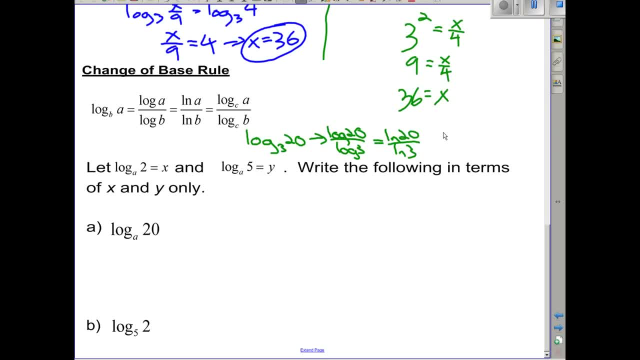 You can't do that And that's not what the question is asking you for anyways, Just looking for an expression in terms of only x and y That represents a number, That's log base a of 20.. Let's think about log base a of 20.. 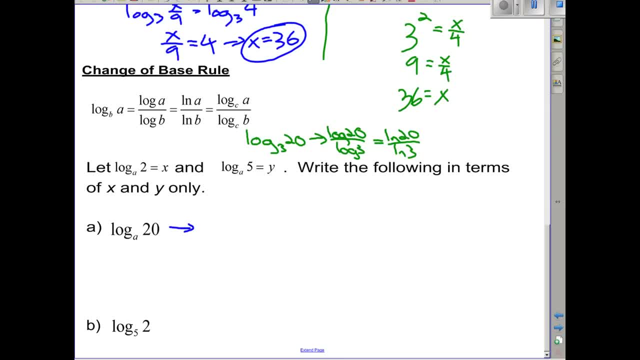 We can split it apart: 20 is 2 times 10.. Or 4 times 5.. I'm going to go with the 2 times 10.. So I could split it this way. That's going to be useful to me, because this part right here is an x. 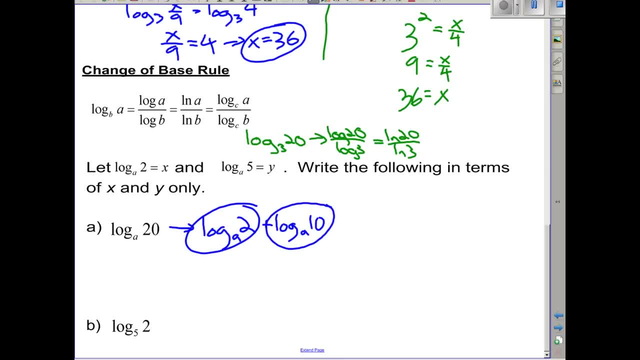 But this part right here doesn't help me at all. Okay, So log base a of 2 plus log base a of 10.. I could split some more though Log base a of 2. And then 10 is the same as 2 times 5.. 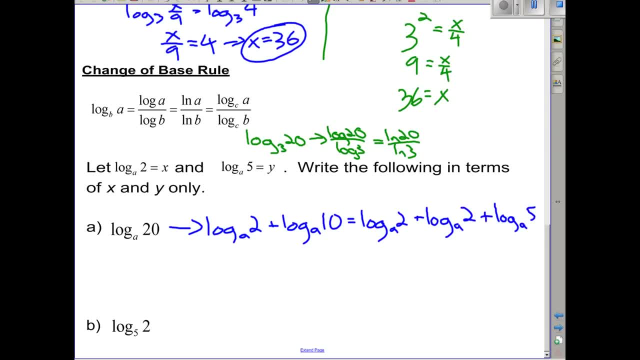 Ooh, So this means log base a of 2 is an x plus another x plus a y. Okay, And there would be a lot of different ways that you could get there. You could have split it to start with as log base a of 4 plus log base a of 5.. 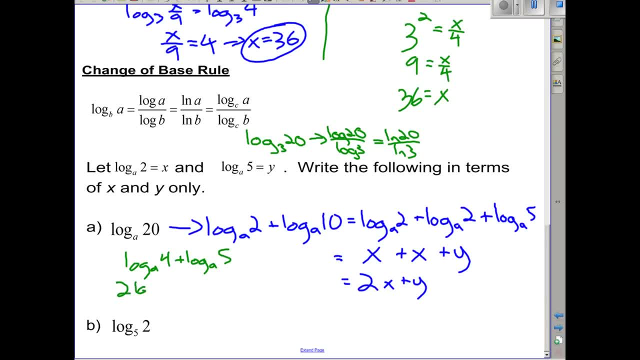 I said 4 is 2 to the power of 2.. So this is really 2 times log base a of 2 plus log base a of 5.. Still going to get you to 2 x's plus a y, Alright. 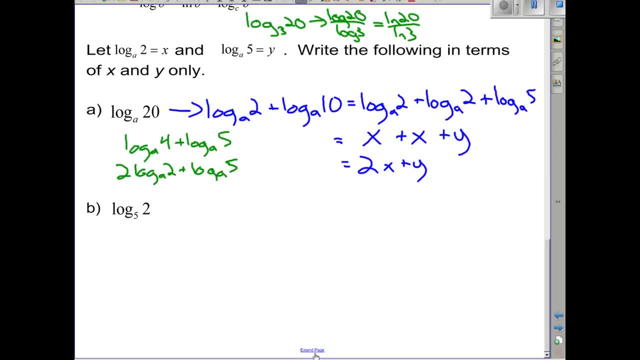 Here's where it gets kind of fun: Log base 5 of 2.. If I wanted to do this in my calculator and just find what the value of that is, I'd probably go: log of 2 divided by log of 5 using change of base rule. 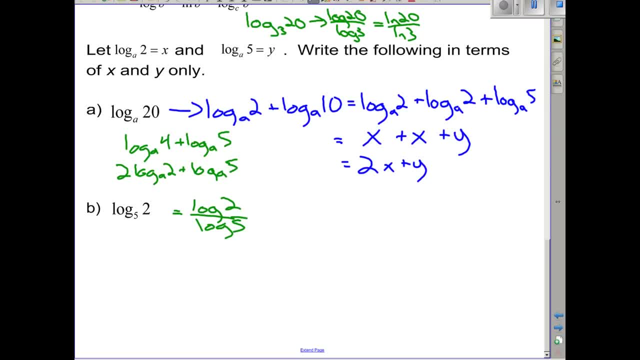 Oh, but that's not what we're being asked for, Not the value of this, but how we could express it in terms of x and y. And here's the little trick: It doesn't have to be log base 10 that we're using. 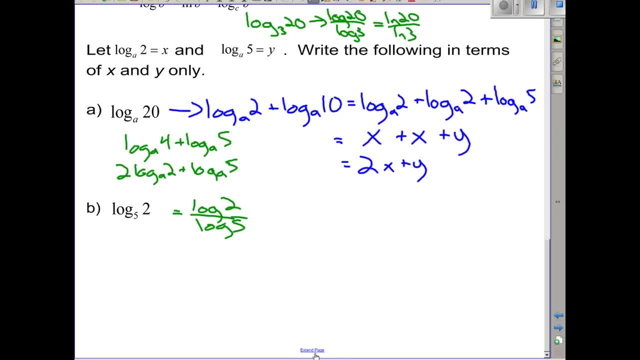 It could be log of any base. What base do we want in this question? Bases of a. So log base a of 2 over log base a of 5. Which is the same as x over y. Pretty sneaky Alright. 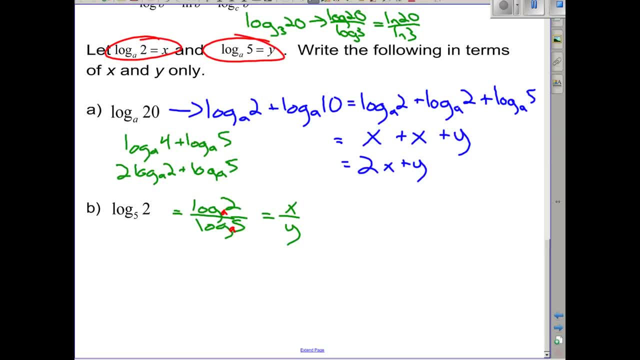 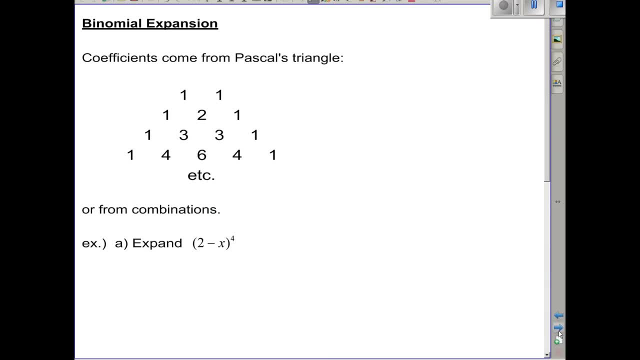 Last topic that's in this sort of mish mash, that's called topic 1 algebra for the SL course And that is binomial expansions. OK, When you're expanding a binomial, your coefficients, or your first set of coefficients, come from Pascal's triangle. 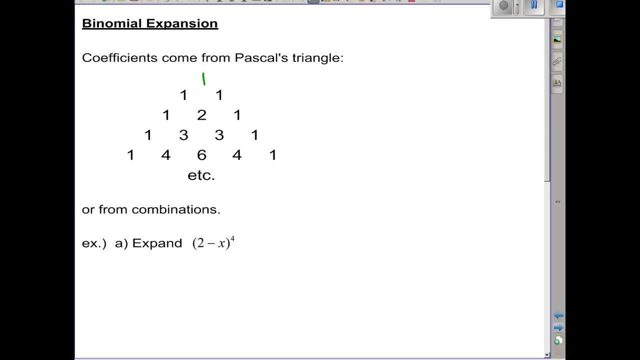 Now I know a lot of people put the first row here of a 1,, which would come from 0, c, 0, 0, 0.. I like to lop it off just for the sake of binomial expansions. 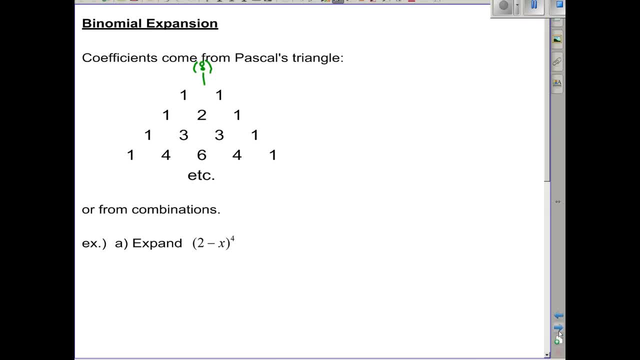 though I will agree, it does not look like a triangle with that first row. So you may have to reconcile the way that you've been taught with having either a first row or not, Or you can think of this as coming from the first row. 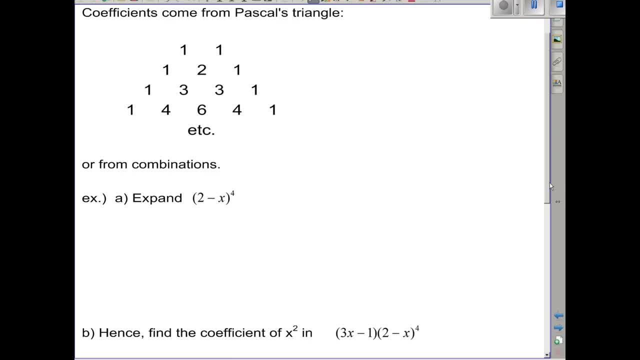 It's coming from combinations. OK, And if we were to write Pascal's triangle in terms of combinations and start at this row with two entries, this would come from 1, c 0, then 1, c- 1.. 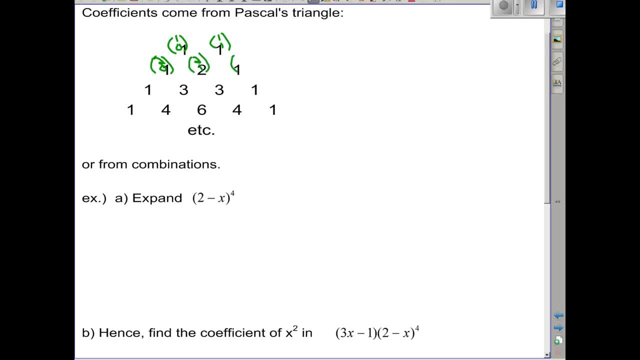 The next row would be 2, c 0, 2, c 1, 2, c 2.. So Pascal's triangle gives you this nifty little way of finding combinations really easily: 4, c- 0.. 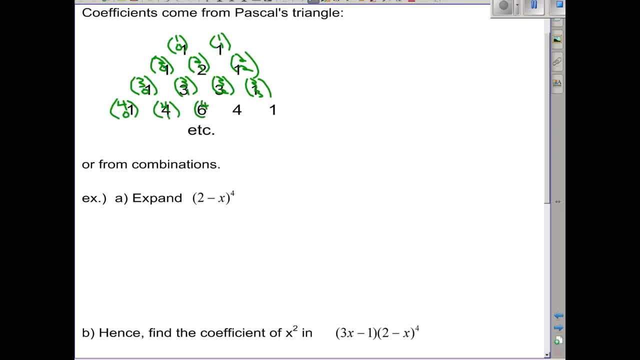 4, c 0.. 4, c 1.. Etc 4, c 2.. 4, c 3.. And just as a point of interest, not that you're going to be responsible for this explicitly- 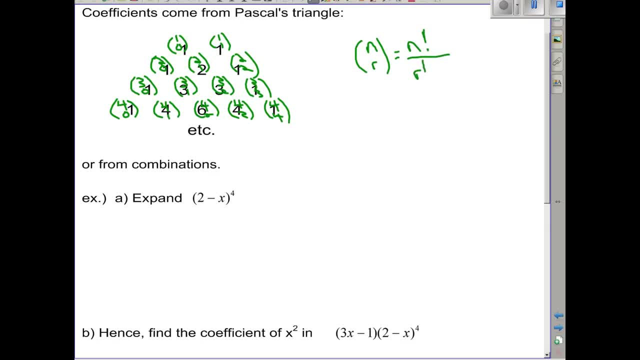 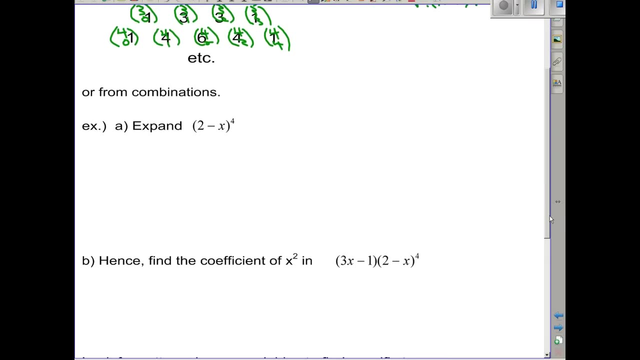 but this is where n c? r comes from. Alright, so if we want to expand 2 minus x to the fourth, here's how I do it. if I were going to actually write down the combinations that are going to be used, 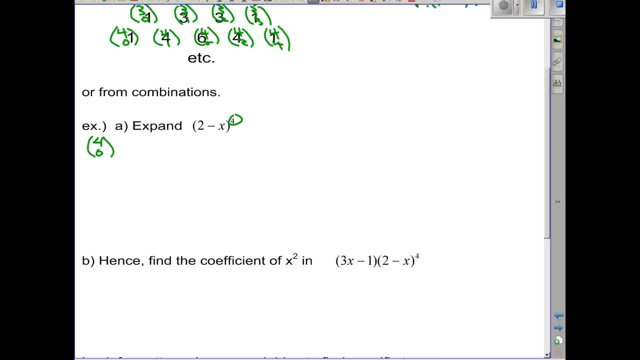 It's to the power of 4, so I'm going to need 4, c, 0 as my first coefficient. I'm going to take the first term in the binomial and raise it to that highest power of 4.. The negative x is going to be raised to the power of 0, so it's not going to show up at all. 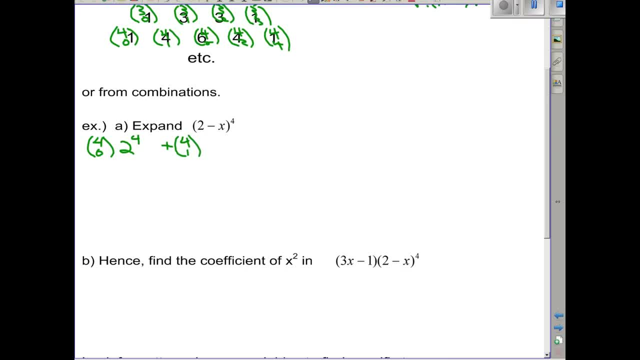 My next term will have a 4, c 1. for starters, I'm going to just write in all the different initial coefficients: 4, c 1.. 4, c 2.. 4, c 3.. 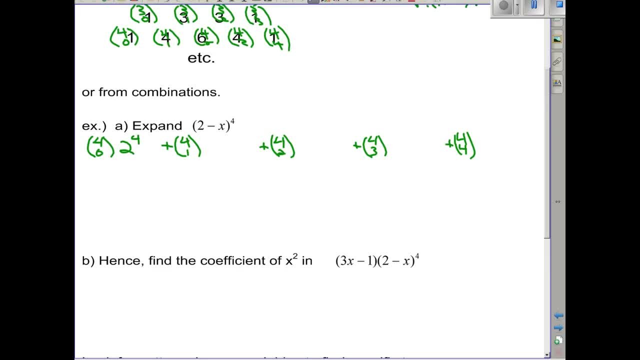 And finally 4, c 4.. I can't have a 4, c 5.. Now, as I go across. initially I had 2 to the power of 4.. Now I'm going to have 2 to the power of 3.. 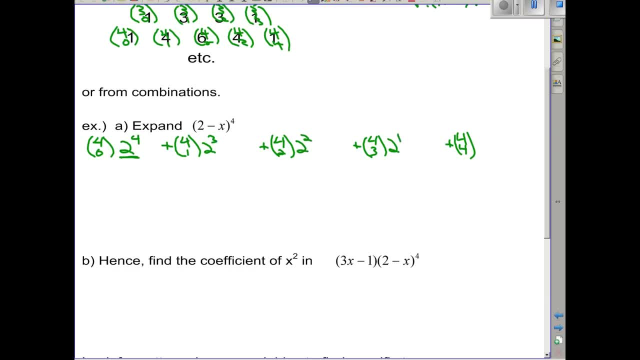 2 to the power of 2.. 2 to the power of 1. And finally, 2 to the power of 0,, which is just 1.. I don't have to show it. See how the powers went down on this first coefficient. 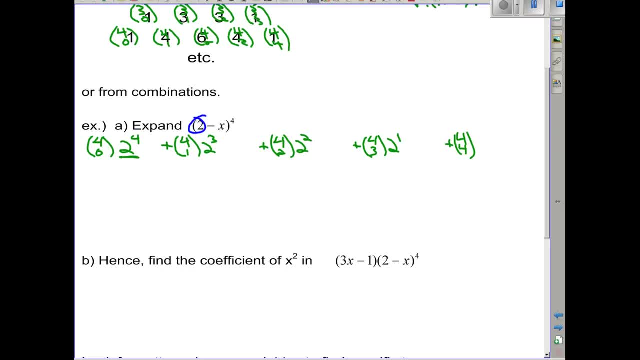 Or this first term in the binomial. rather, Now we're going to take the second term and its powers are going to go up. We're multiplying here, So this will be times negative x, Times negative x- squared Times negative x- cubed. 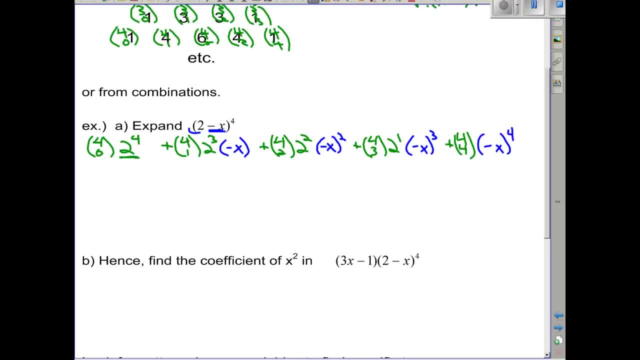 And finally times negative x to the fourth. So powers go down on the first term in the binomial, Powers move upwards on the last term in the binomial. You may not have wanted to show this first term, To show this first step with the combinations. 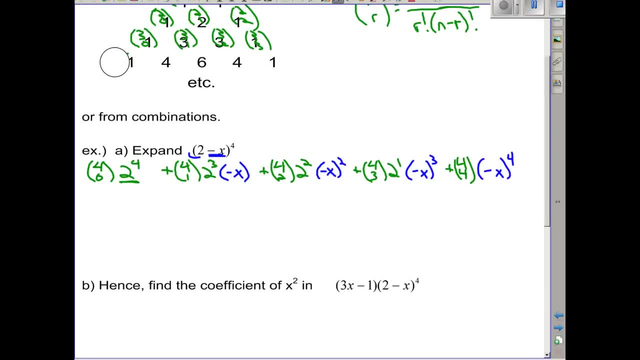 you might have gone straight to Pascal's triangle and said power of 4, that's the fourth row of the triangle, if I write it without that first top number. So coefficients of initial, coefficients of 1,, 4,, 6,, 4, 1.. 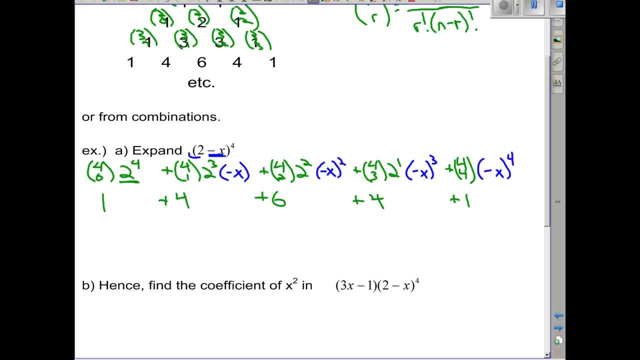 Or I could go to my GDC and get it to do 4, c, 0 for me, etc. 2 to the fourth I know is 16.. This will be 2 to the third. That's 8 times negative x. 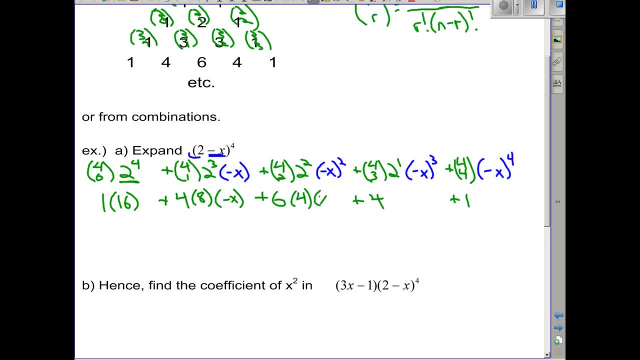 2 squared is 4.. I'm just working out each individual part here, Working out the exponents and the combinations: Negative x, cubed, And this will be x to the fourth. Okay, let's multiply: 1 times 16 is 16.. 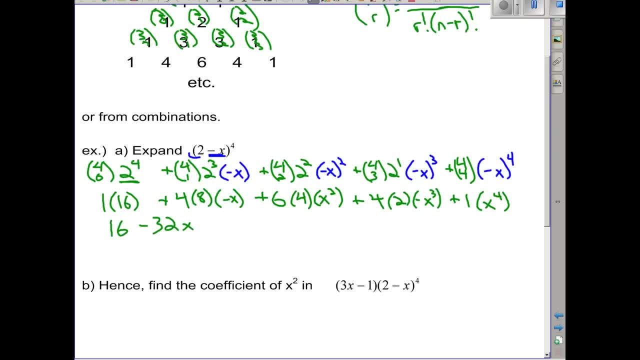 Minus 32x Plus 24x squared, Minus 8x cubed And plus x to the fourth, There's the expansion. Alternately, we could have written out 2 minus x 4 times. Use distributive property. 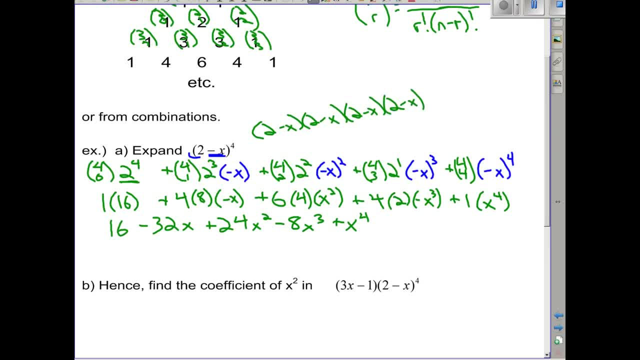 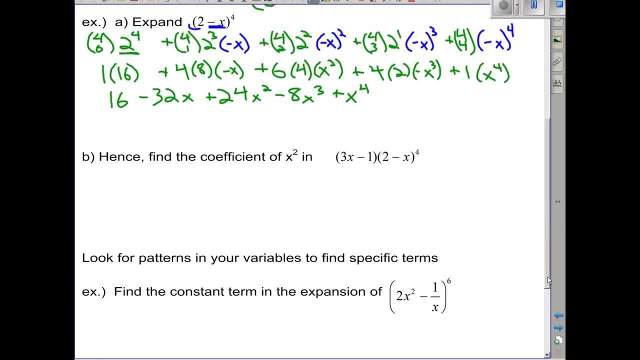 Really that's going to be unpleasant, And the likelihood of following it through without any errors is relatively low. So binomial expansion can really save us some time, And especially being able to use the triangle well. Hence find the coefficient of x squared in this. 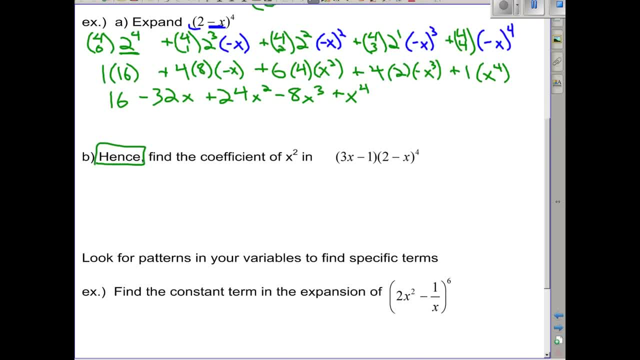 Alright, notice the hence. It means using what we just found. So 3x minus 1 times. Oh, I already know what 2 minus x to the fourth is. It's this. Now, where am I going to get x squared? 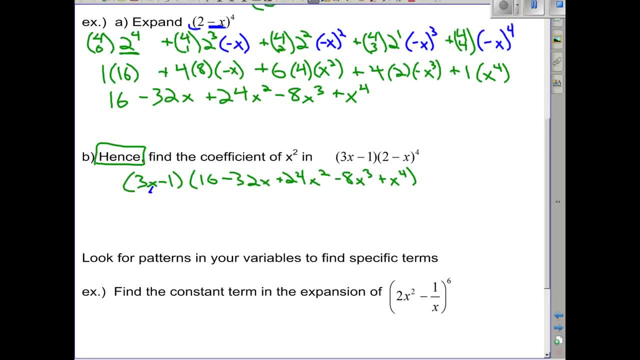 Well, I'll get x squared from the 3x part times the x term in here And also from the negative 1 times the x squared term. So that's going to lead us to 3x times negative. 32x is negative, 96x squared. 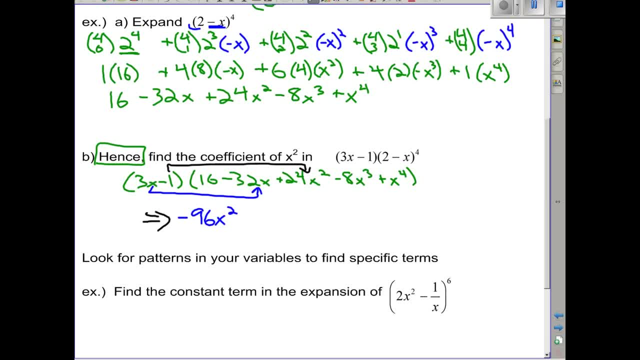 Negative: 1. Times 24 is negative, 24x squared. I don't have to do the whole expansion to figure out what the coefficient of x squared is going to be. I could, but it would be a waste of time And, as you know, time is at a premium in these exams. 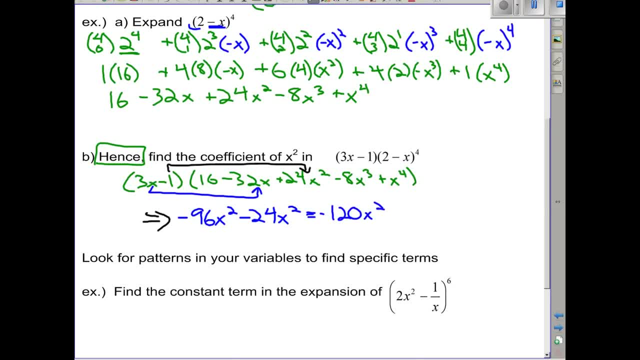 Gives us negative 120x squared And sadly and somewhat cheaply, that probably isn't going to get you full marks. You have to make sure that you answer the question that's being asked. It's only asking for the coefficient of x squared. 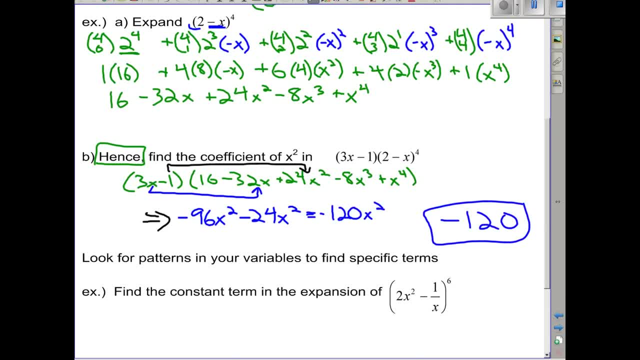 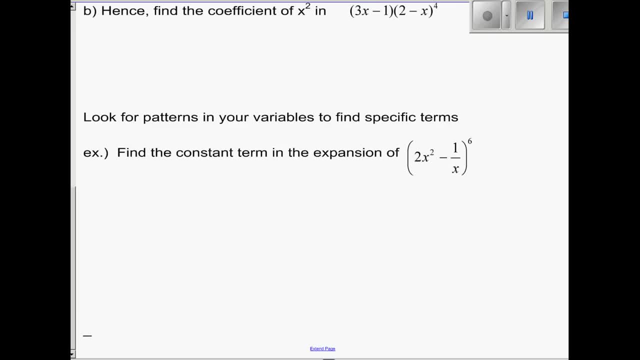 So the coefficient is negative 120.. Sometimes when we're looking for specific terms in our expansions, we'll want to look at patterns that appear on the variables. So let's take a look at this one. Find the constant term in the expansion of 2x squared minus 1 over x to the power of 6.. 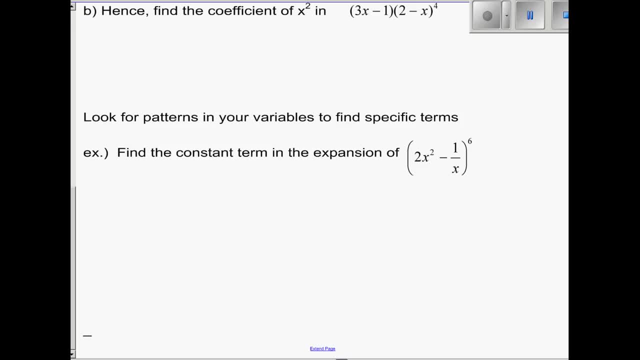 There is a formula for finding a specific term in an expansion, But what I like to do is just write out the pattern And everything sort of takes care of itself. So my first term would be a 6c0.. It's got 2x squared, all to the power of 6.. 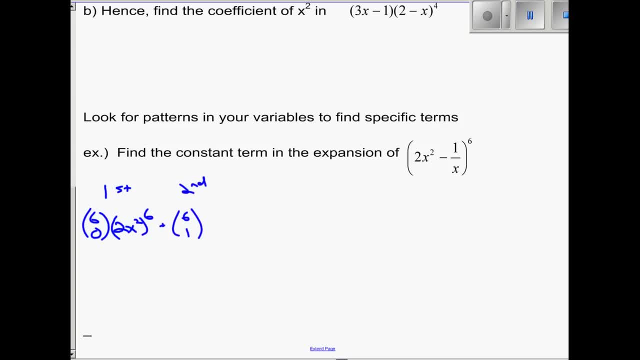 My second term would be a 6c1.. It would have 2x squared all to the power of 5. And now I'd have negative 1 over x. If I look at what's going on here, my first term's going to have an x squared to the 6th. 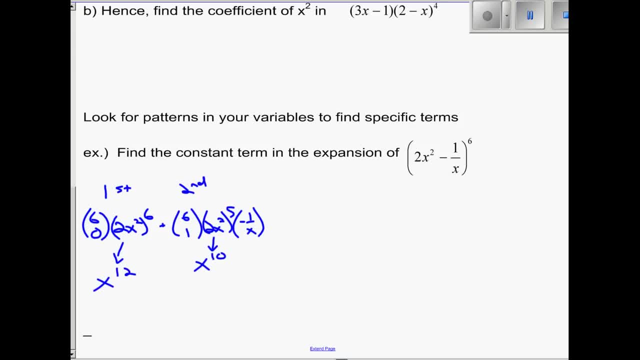 Or an x to the 12th. My second term will have an x to the 10th times negative 1 over x. In other words, it'll have an x to the 9th. That pattern of powers decreasing by 3 is going to continue. 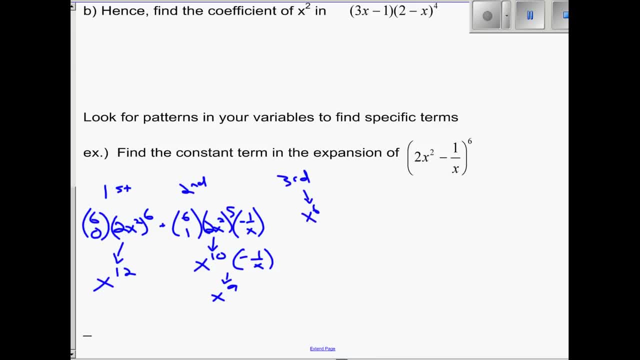 So my third term would give me an x to the 6th, My fourth is going to be an x to the power of 3. And my fifth will give me x to the power of 0. Ah, which means a constant term. 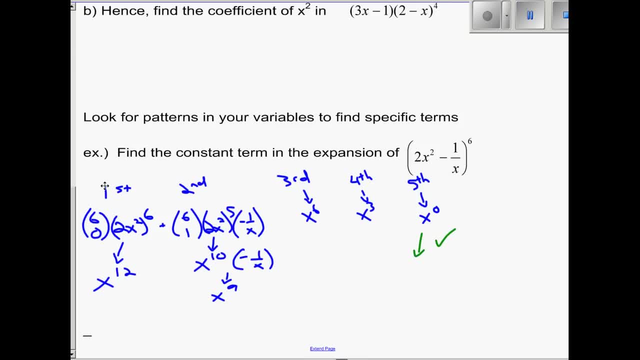 So this is the one that we want. Let's set it up. First term had 6c0.. Second had 6c1.. Third would have 6c2.. Fourth would have 6c3.. Fifth would have 6c4.. 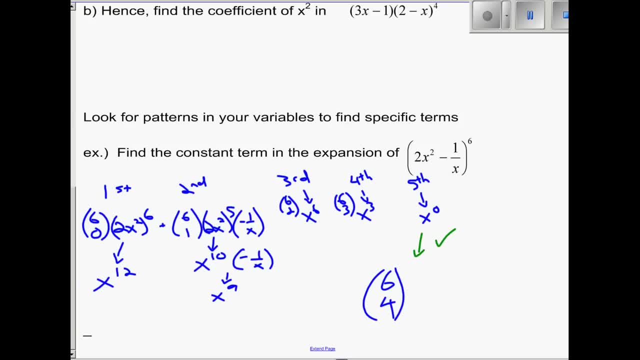 And obviously you don't have to write out all this sort of rough work that I'm doing. It can be happening in your head. Okay, the first term had 2x squared to the power of 6.. Then we'll have 2x squared to the power of 5.. 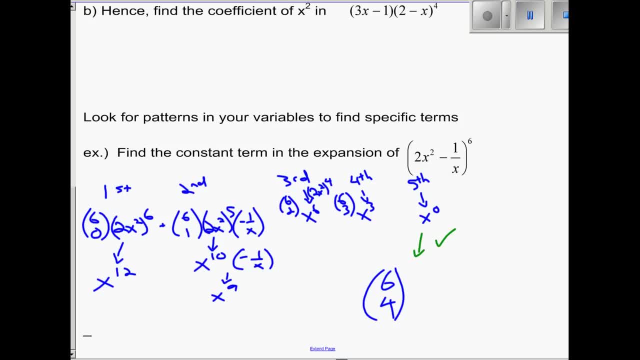 Then 2x squared to the power of 4 in the third term, To the power of 3 in the fourth term, And 2x squared all to the power of 2 in the fifth term, Our negative 1 over x makes its first appearance in the second term.